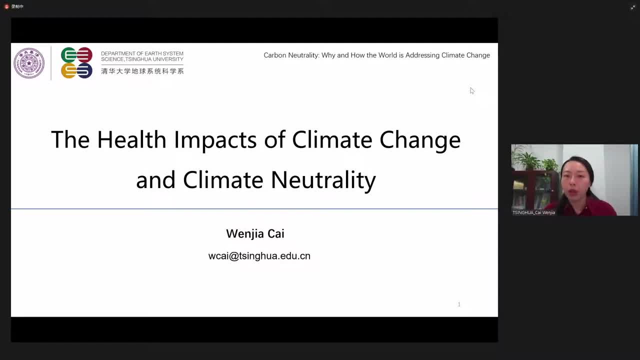 And I would also encourage you to type in your questions into the chat box. And I would also encourage you to type in your questions into the chat box, And I would also encourage you to type in your questions into the chat box. So carbon neutrality is something we are really keen to explore in our projects. 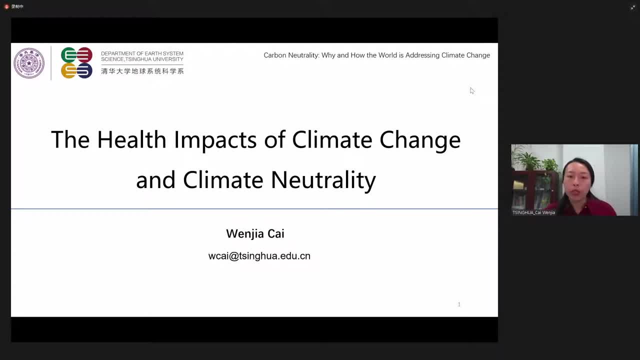 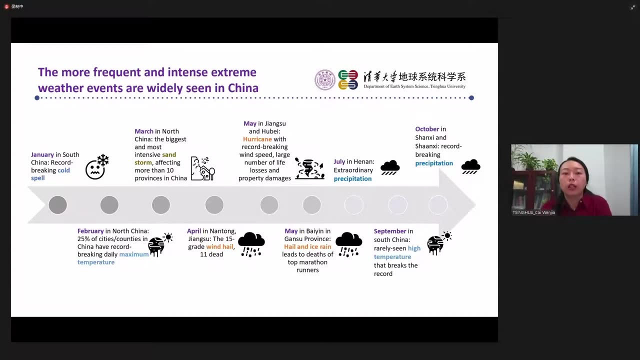 And so today I'm going to take you through the health impacts of climate change and the carbon neutrality, And I apologize that I only have this graph for China, But I believe most of us today can see more frequent and more intense extreme weather events that are happening all around the world. So let's just take China, for example. We have this: 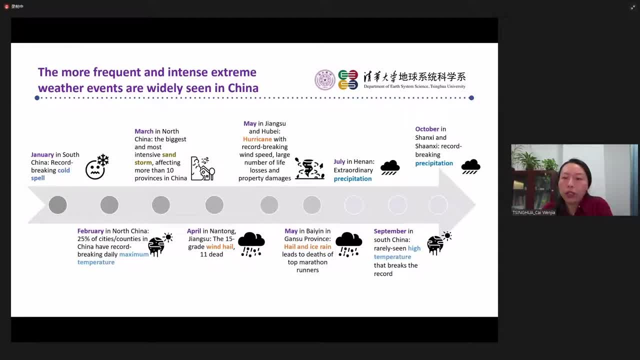 in January in South China, those record-breaking cold spell, And actually this year a lot of people are worrying whether we will have an extremely cold winter in December or in January. So we are starting to worry about those upcoming extreme weather events And that's something. 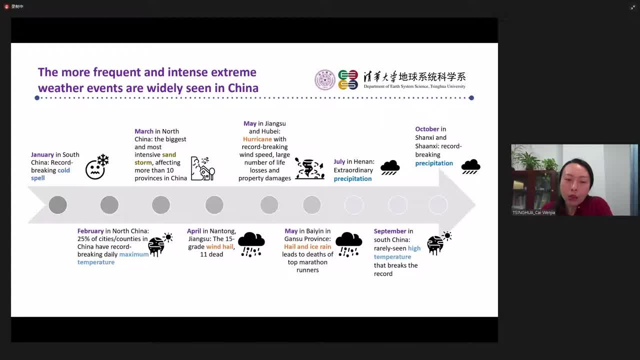 that's something never happened before. And also in February in north part of China, where it used to be very cold. about one quarter of cities in north China have those record-breaking daily maximize maximum temperature, which means they never had such high temperatures before. And also in March, if you remember, we have this sandstorms in north. 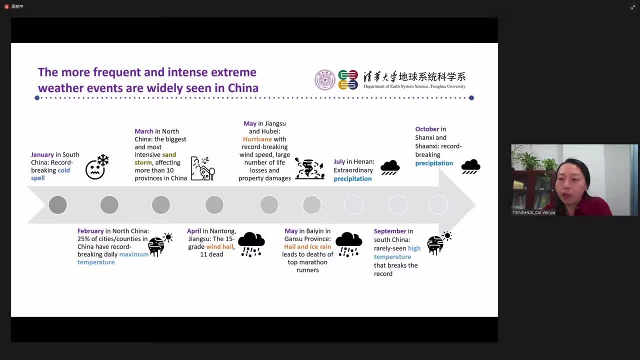 part of China, affecting more than 10 provinces and billions of people, And also in well, if you remember, also in May, we have this marathon games In Gansu province, And when these top runners are were joining this marathon games, they met with this. 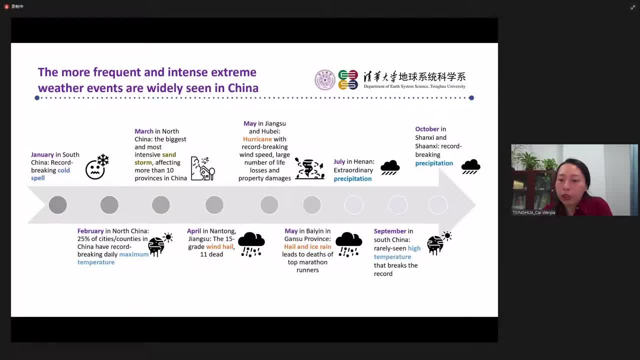 extreme hail and ice rain and which leads to the deaths of more than 20 people, And they are almost the top marathon runners in China And which is really sad. And if you live in China, you can't miss the July, the biggest news. 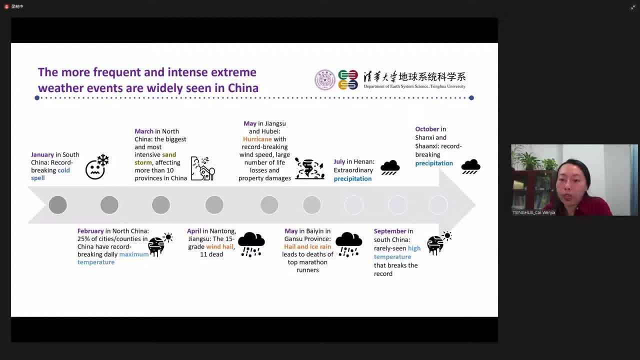 In July, which is the extraordinary precipitation in Henan provinces. They said it's like a once in a thousand years rainstorm, So the whole city and actually several cities in Henan are just buried underwater. And also and also after that, we've also seen like record-breaking precipitation in 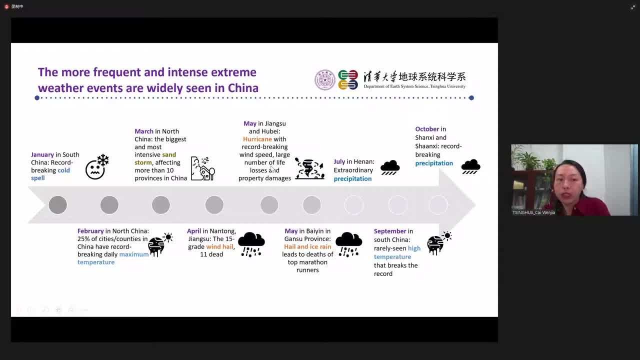 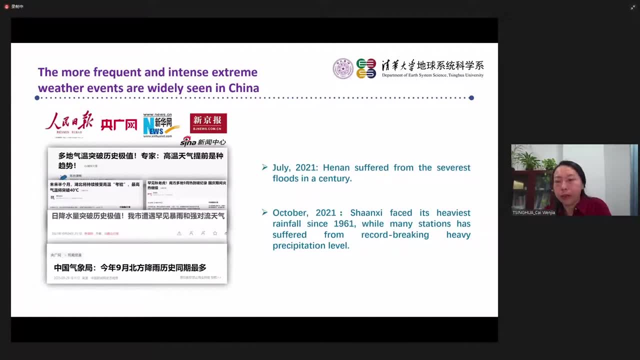 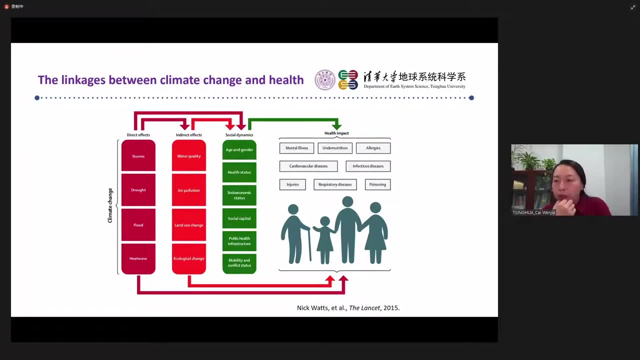 Shanxi and Shanxi province. So you can see there are a lot of news focusing on this intense extreme weather events in China. And what, what? what are these? like temperature change and also the extreme weather events relate to us, I think most of us, I mean everyone, everyone on. 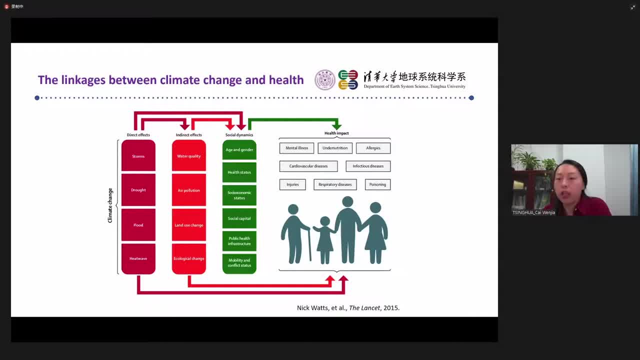 this planet. they care about the health of themselves and as well as their parents and their children. However, you, although most of us, are thinking that our health are determined by, like the food we take every day and the exercise we take every day, and even the mood we have, whether we have good friends and good working environments, But a lot of people don't. 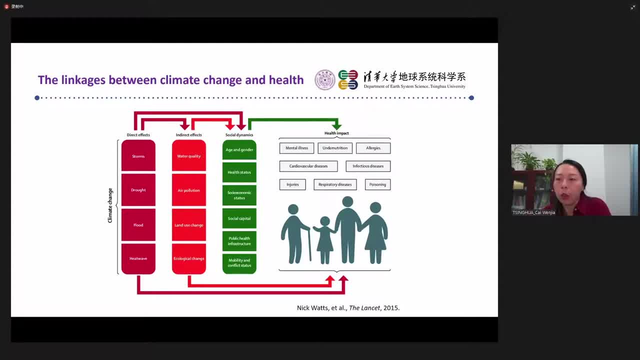 recognize that climate change is actually affecting each one of us health from various ways. So you can see from this graph- and this is a graph which was published in The Lancet, which is the most prestigious medical journals in the world right now, So it was published in 2015,- which summarizes the direct and indirect links between 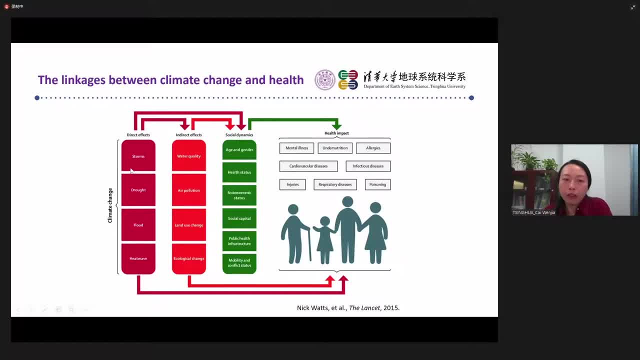 climate change and health, And you can see from this graph what are. the phenomenon of climate change is that we are having more and more and intense storms, droughts, floods and heat waves in everyday life, And these meteorological phenomenon will have the direct 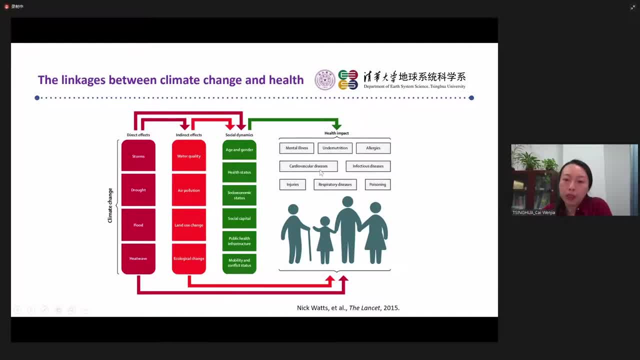 effects on the health. For example, some people would have their well incidence, more incidence of those effects. So, for example, people would have their well incidence, more incidence of the those effects of the �Book. But we don't. we do have the direct effects and drive more on the. 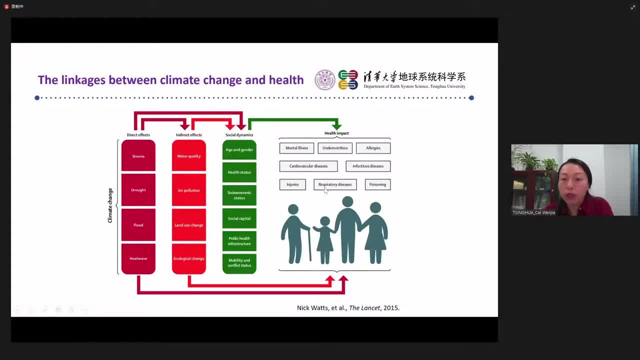 cardiovascular diseases or respiratory diseases. And these are the direct effects. And if we look at the indirect effects, we know, for example, air pollution is a serious environmental problem faced by many countries in the world And actually climate change has an indirect. 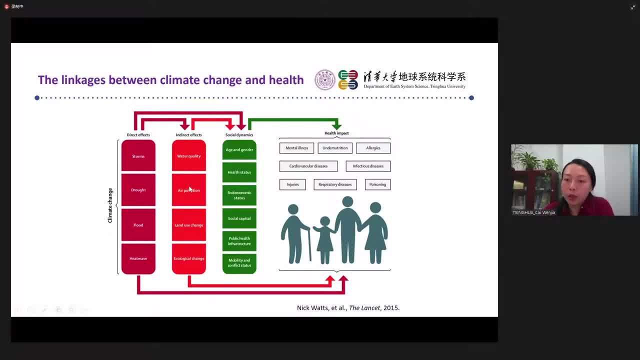 effect on air pollution Sometimes, while most of the existing literature says that climate change will lead to more stabilized atmosphere in the future. So even if we emit the same amount of air pollutants, we will have much severe air pollution. So that is why it will also climate change like. 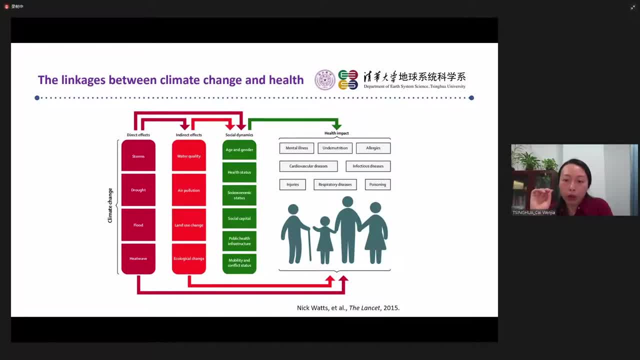 will act like an invisible hand and will jeopardize our health from different ways. And another thing is ecological change. Probably most of you, or some of you, are not familiar with ecological change, But if you look at the spatial distribution of mosquitoes, you would see the trend. 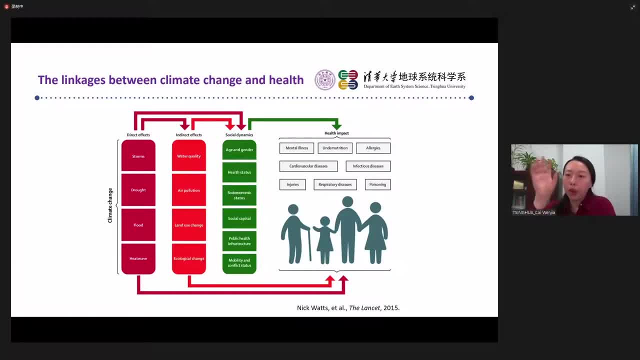 a very clear trend that mosquitoes are moving north and their survival duration during a year has been extended. So, for example, in Beijing you would probably still see a mosquito in November, and you would- you could imagine to see a new mosquito from like April or even earlier. 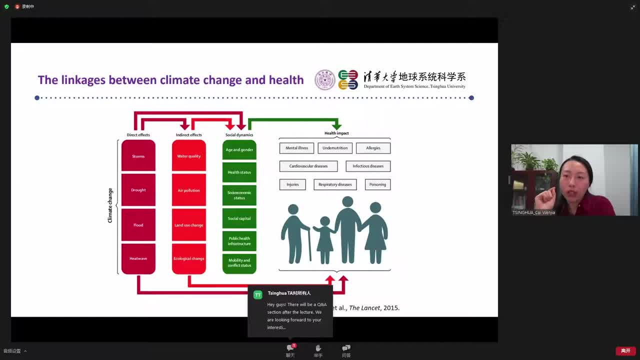 in Beijing. So supposing that we are living, or actually we are living, in this warmer world, And can you imagine that in Beijing we will meeting with those annoying mosquitoes for all, all around the year. So that is something we are expected to see in the future. 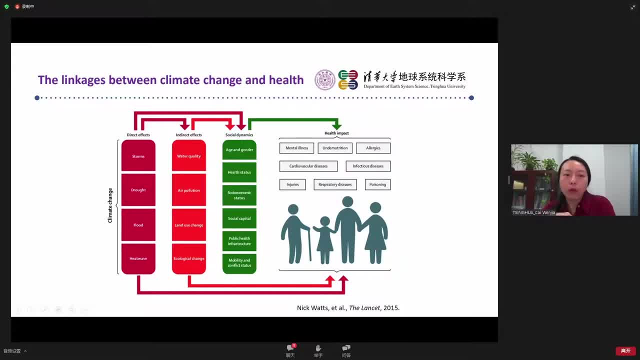 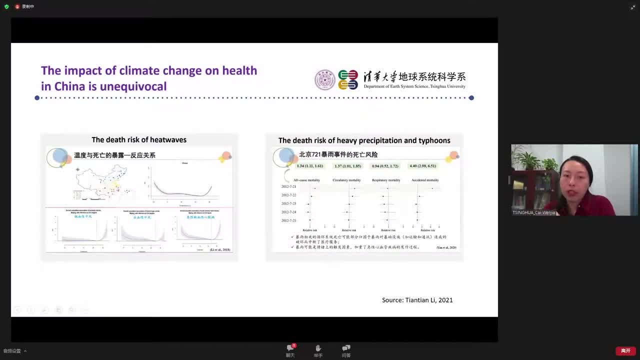 So I am here. I am showing some of the graphs on the statistics or the real data. In the middle of the slide I have a graph showing the most recent data. that shows the most recent data For the impact on climate change on health in China. the left figure shows the death risk of heat waves. 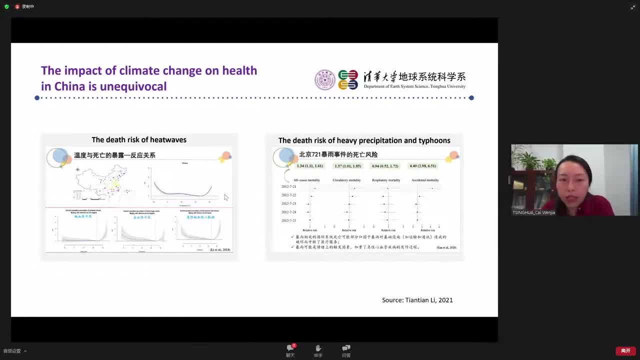 And if you look at this curve, this U-shape curve, the horizontal axle means the temperature, So it starts from minus 10 degrees to Celsius degrees, to more than 30 degrees in China, And then the vertical exo means the relative relative risk of death. so the higher the rest, uh, the relative risk of death. 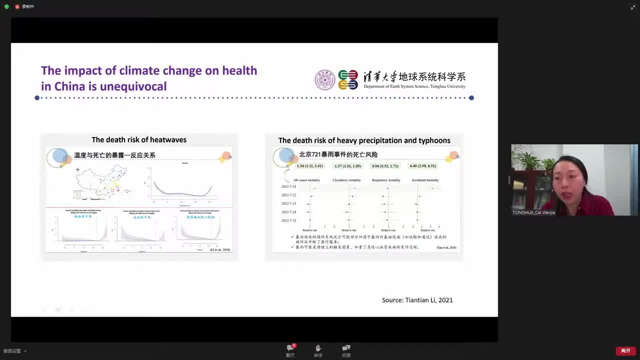 is. there is a more, there is a higher possibility for those vulnerable people to meet with problems that has a life issue, so that that actually damage uh leads to the death of these people. so if you look at this graph, this looks like a u-shaped uh curve, and what does it mean? 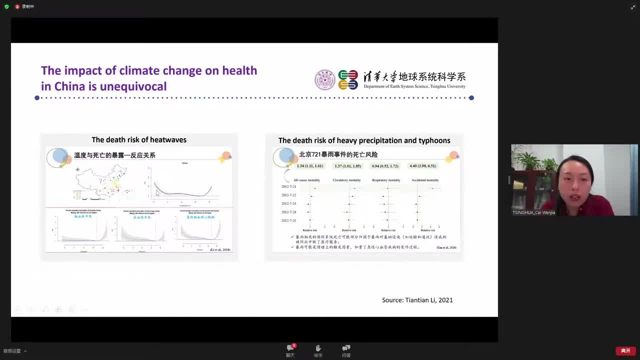 it means that the lower the temperature is, the higher the desk risk is. and also, if we look at the right part of the curve, the higher the temperature is, also the the higher the um the death risk is. so if we go, uh, we, if we're aiming for like a warming world, 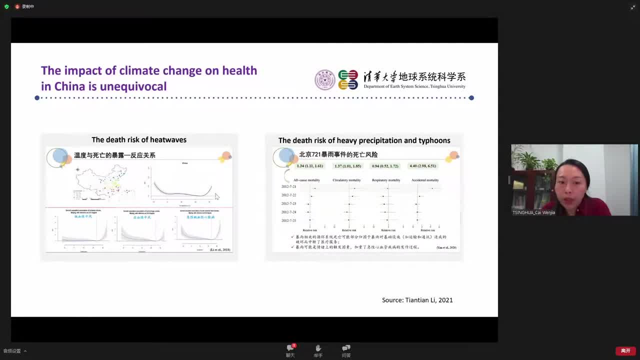 we will see more temperatures, uh happening in this part of uh area and we will have less cold events, although sometimes we still have this cold spell, which means the the the weather is extremely cold, but you see the curve. this right part is rising more rapidly than the left part, the cold part. 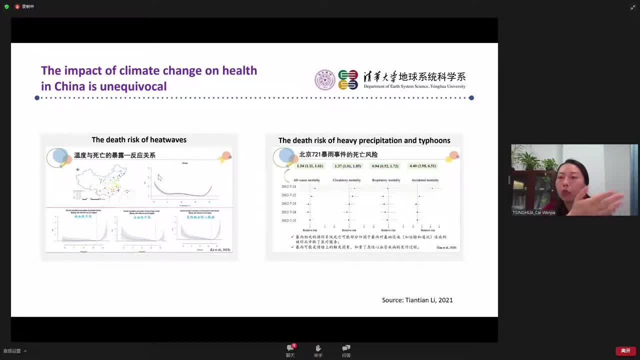 so that is why, if we're combining, like the less cold- uh cold related deaths and the more uh death- heat related deaths, the the warming world will actually lead to more temperature related deaths, and the right figure actually shows the death risk of heavy precipitation and typhoons. 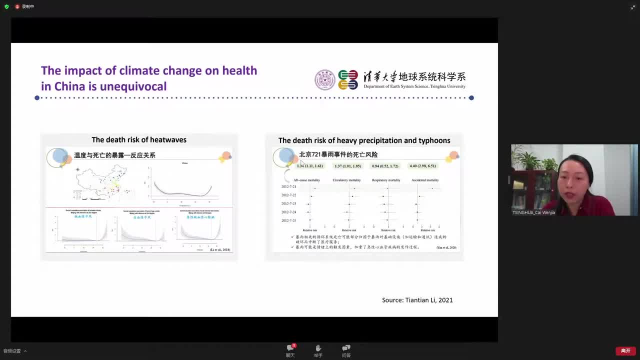 and this is a gra. this is a graph showing the death risk. uh in uh. beijing, uh in um- i can't remember which year it is, but it's. we had a like a uh also uh, once in a hundred years- precipitation which leads to uh 60, more than 60 people's death. 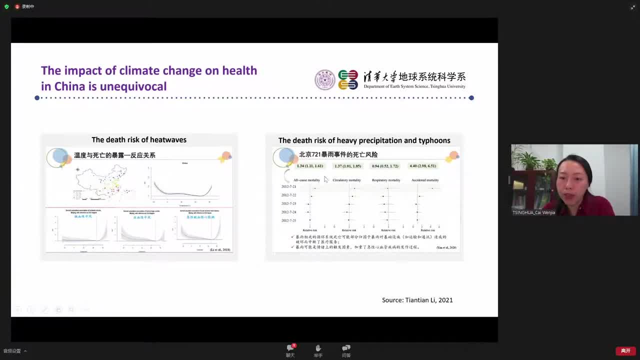 and then and during that heavy precipitation event, we will see there or there are a very obvious increase in the accidental mortality and also the other some of the other mortality rate are also increasing rapidly. so the the key messages from these two figures is that the impact of climate change on health is unequivocal. we have a lot of evidence to 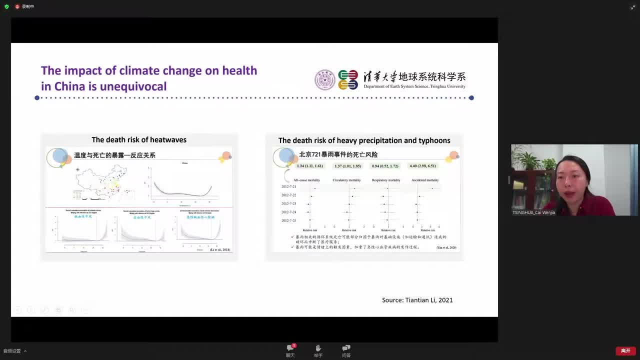 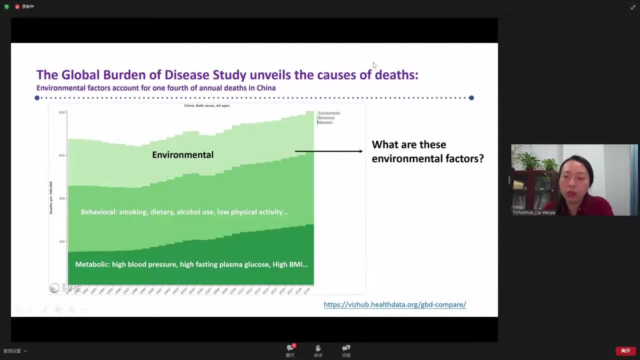 show that climate change has a serious impact on health. and if you still don't believe, from those single graphs, let's come, let's, let's see this: uh, global burden of disease studies results together. you know, global burden of disease is a like a. it's like a giant project which combines the efforts. 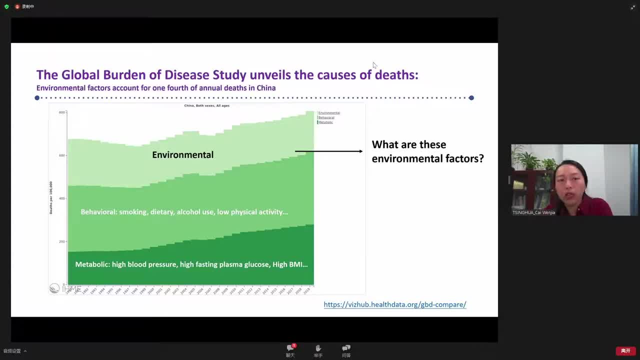 of more than 1 000 scholars around the world. so what is the global burden of disease? it actually shows why are- uh, why are the people in, in in a certain country is dying from? so, for example, in china, we have a lot of people who are dying from diabetes. 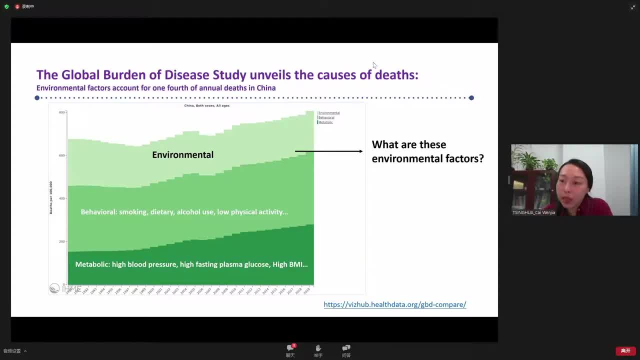 from lung, lung cancer, from stomach cancer. a lot of these kind of factors are leading to the death of people. so this graph actually shows the several categories of deaths, of factors that lead to death. so you can see a lot of people actually are dying from the metabolic reasons. for example, they 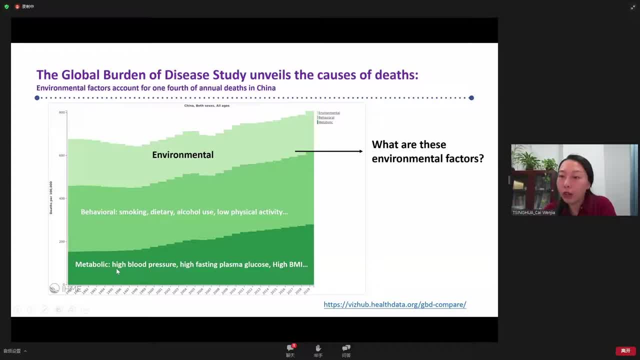 have high blood pressure, they have high bmi, or meaning they they are too fat, have obesity problems. and the second reason, or the largest reason, because they are having behavioral reasons. for example, if they are smoking, they have a higher risk of dying. and also the alcohol use and, like you, have a not very healthy diet and for a lot of 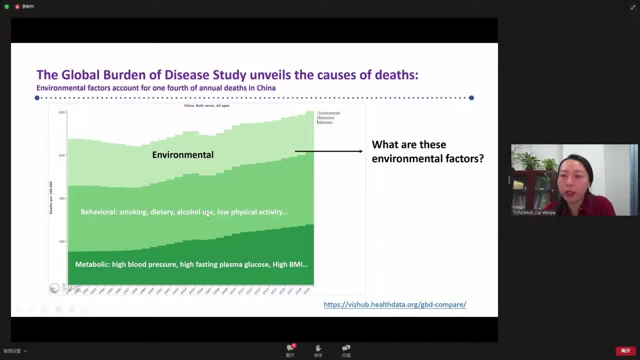 the well, students, or a lot of the people at the working age. they are lack of physical activity, and these are all leading to the deaths of Chinese people, and these are something that these two green, greener parts are something we're very familiar with. however, if we look at the light, 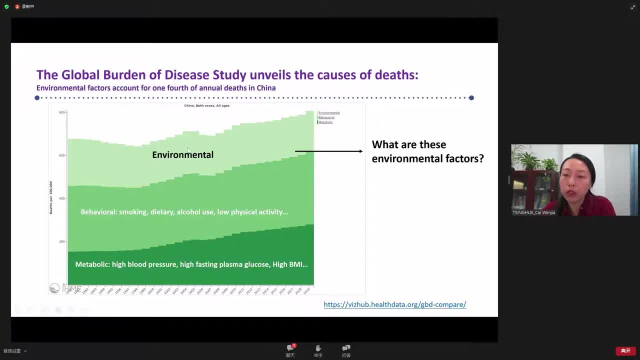 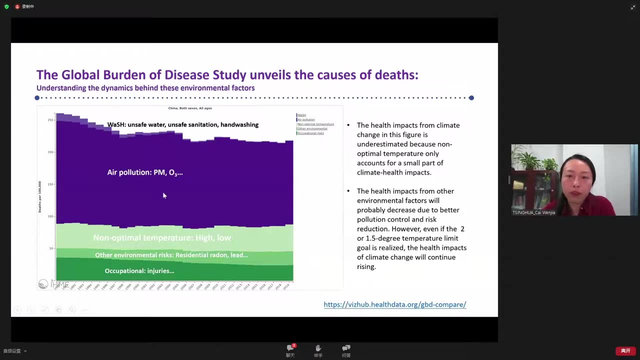 green part, which is the environmental part. I don't think a lot of people are familiar with that, so let's together see how. what are these environmental factors? and you can see from this of the those environmental factors. so, among all the factors, that belongs to the environmental. 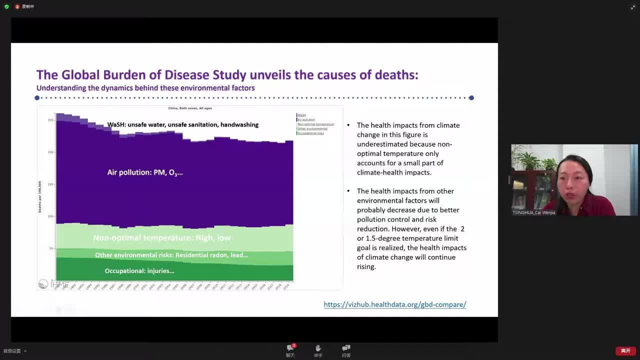 factors- air pollution- that we are most of us are familiar with- are contributing the most. so we about air pollution- we are referring to the particular matter pollution and also the ozone pollution. well, so these are something that we are familiar with, but let's look at the second largest part, which is the non-optimal temperature. that is something I 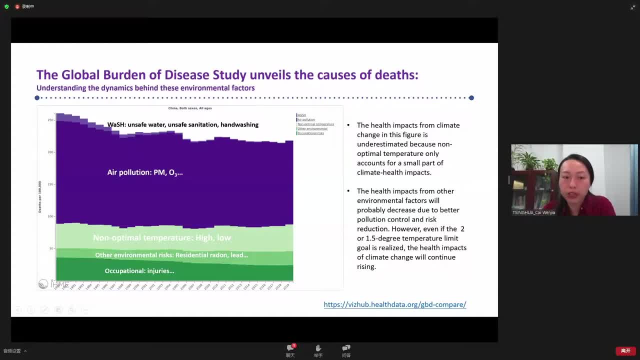 just explained in the u-shaped curve. so if, if the temperature is very low or is very high, we call it the non-optimal temperature. so this part actually are taking up a relatively large share in the total death risks of environmental risks. so this part- well, this part already takes up like a quarter of the of the whole deaths. 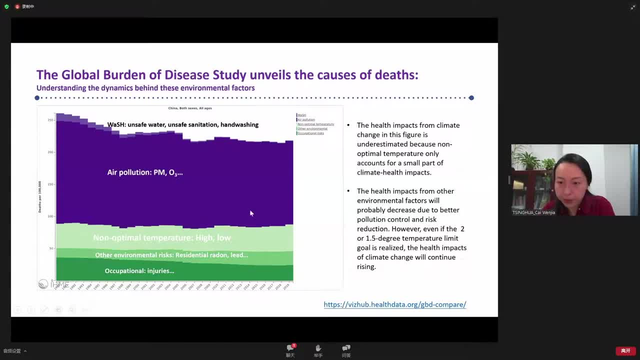 in the environmental related deaths and if you, if we look at this figure from a dynamic point of view- I don't know well how many of you are living in China, but if you live in China, you can, you can feel this vividly or from your just. 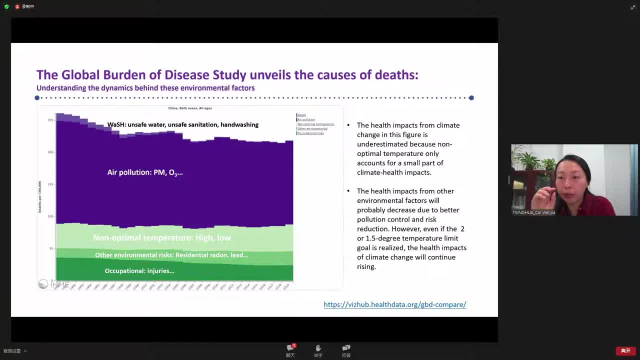 from your eye that the air pollution in China is improving a lot and we are having more and more blue skies every year. so if dynamically, I would say, the burden, the health burden- from the air pollution is going down, however, the non-temperature, non-optimal temperature events, 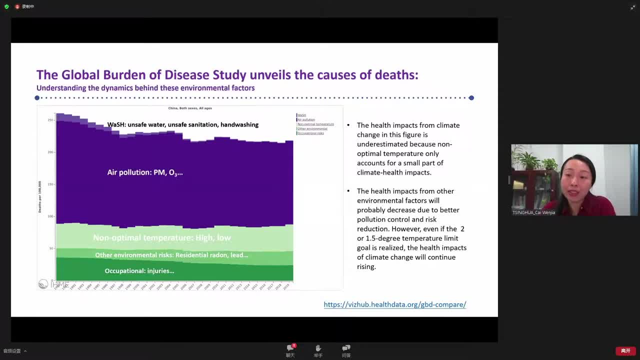 they will be. the days that we have this non-optimal temperature will be like more and more than what we had before, because we are having this global trend of warming and it is not like the air pollution that China can determine the trend of the improve, improvement or the rate of the. 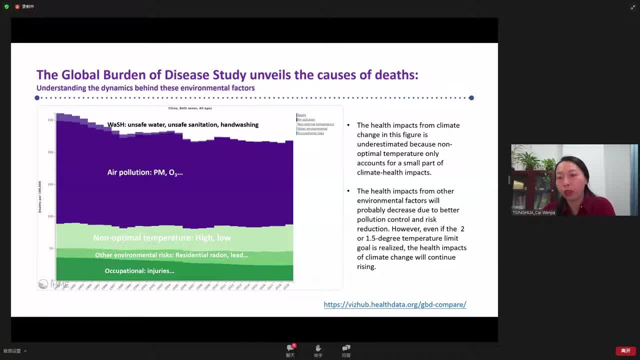 improvement. the temperature thing is like a global issue. it can never be decided by one single country. so it's like a joint efforts for a foreign country to determine the trend of the air pollution from the from the world. so if we don't achieve, like the temperature rise limit goals in the Paris 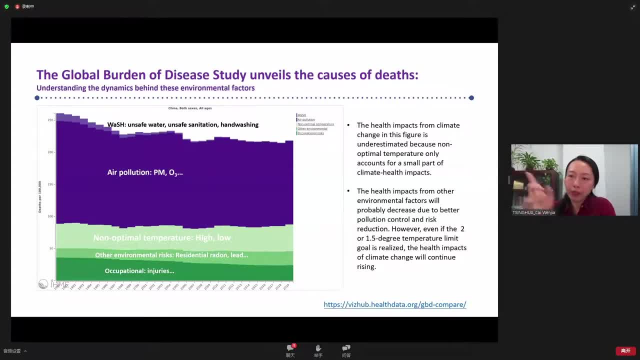 agreement, we will have a soaring which is rapidly increasing temperature in the future and you could see and you could imagine that this part of the health burden will increase in the future and actually the point I made here is that those non-active, non-optimal temperature is only a small part of the health impacts of climate change. just like, just as I, 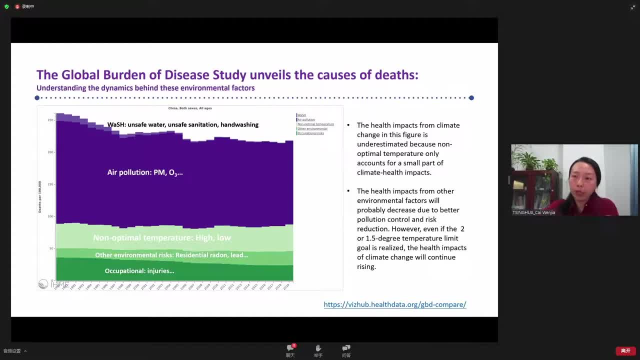 mentioned in in the previous graph. so climate change is actually affecting our health from many different ways. so these graphs are actually underestimated the health impacts from climate change, and that is why we should really think, or or take this issue seriously and to to give more focus to the health impacts of climate change. 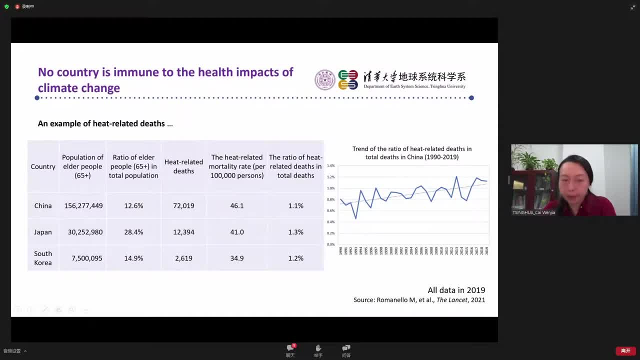 here I see some country-level comparison. if you look at china- I mean if you look at china- we have more than 10 or 12 percent of people who are already, like, defined as older population, and in Japan the aging rate is much higher than before. but if you look at climatology cases, the rate of aging is far higher than that of that, the save normal population, samhih. 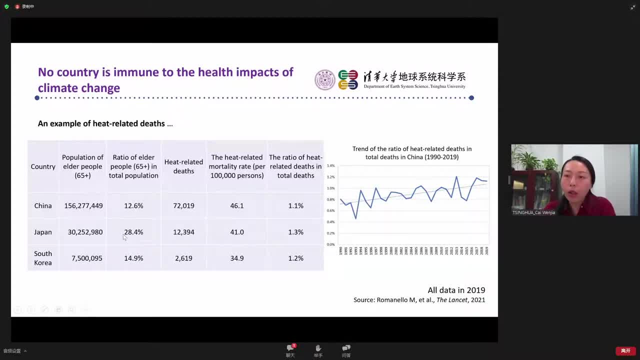 than the other country. they have like one third of people population who are over 65 years old And in South Korea, the aging ratio is a little bit more than the China, China's- statistics. However, if you look at here, if you look at here the ratio of heat related deaths in total deaths, 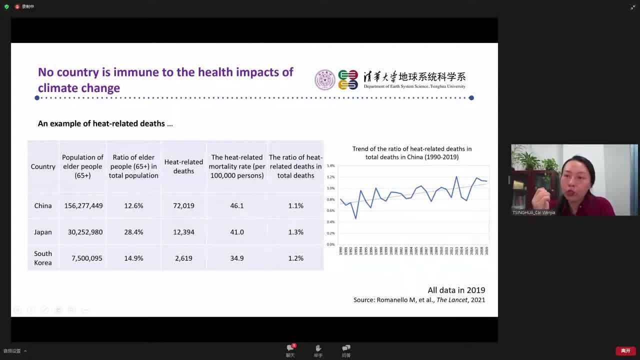 it means that among each 100 people who died this year, around 1% of the total deaths are related to heat. It doesn't mean that they live in extremely hot events and they are too hot, And that gives like immediate deaths of these people. 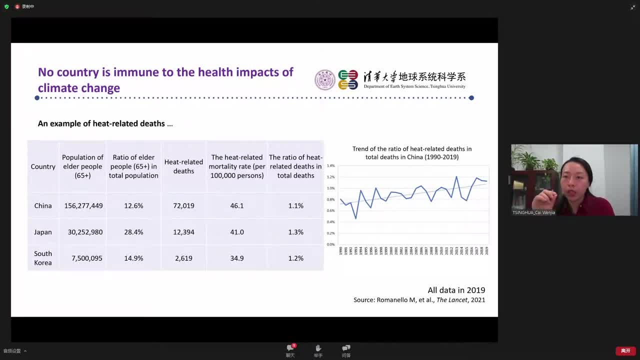 These people are usually having those preconditions in their lives. They have some existing health problems like the cardiovascular disease or some respiratory diseases, And heat's just like a catalyzer for the incidence of these kind of diseases. So around 1%, or more than 1%, of the total deaths are heat related deaths. 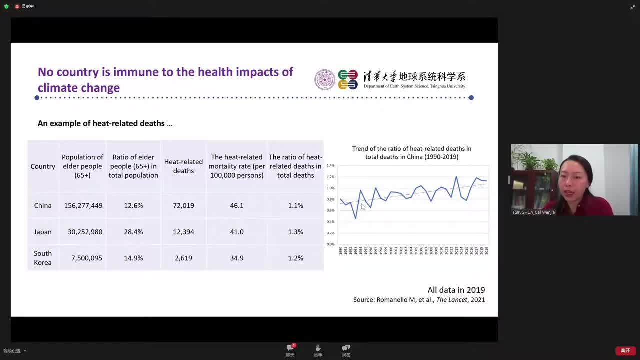 And if we look at this figure, you can see the ratio of heat related deaths in total deaths in China are increasing, Although it's fluctuating every year, but it's increasing steadily. So this actually echoes what I just mentioned, that the health impacts of climate change will keep increasing. 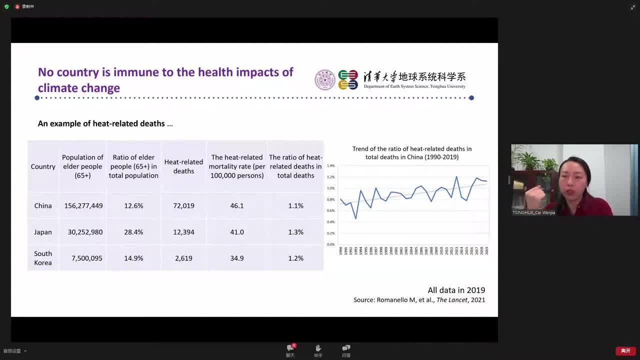 if we don't stop the current climate change trend. So in one sentence I mean: no country is immune to the health impacts of climate change, No matter It's rich country or it's poor country, no matter It's some country, inland country or some any country that are located in along the seashore. 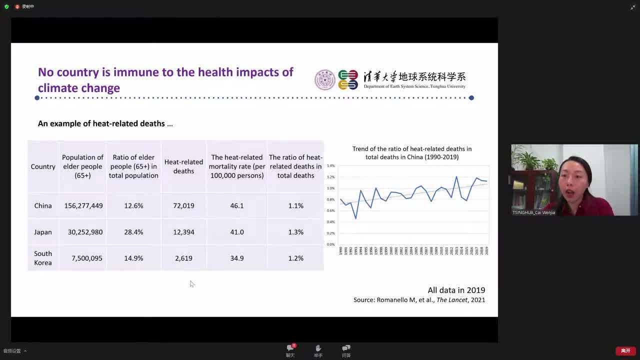 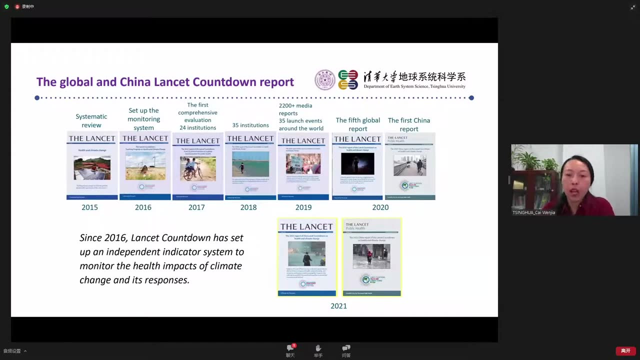 So different countries are facing with different kinds of health threats, And that leads to the introduction to a series of flagship publication on the health and climate change issue, which is the Lancer Countdown Report. I have the honor to join The Lancer Countdown Report since 2015, and 2015 is the time that we have this systematic review on the global trend of climate change impacts on health. 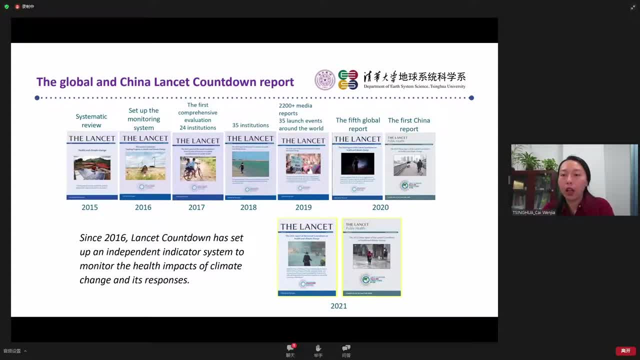 And since 2016,, we actually set up an indicator based monitoring system that tries to monitor the health impacts of climate change and its responses. by responses, We mean the mitigation action and adaptation Action, which I believe you already know, some from the previous lessons. 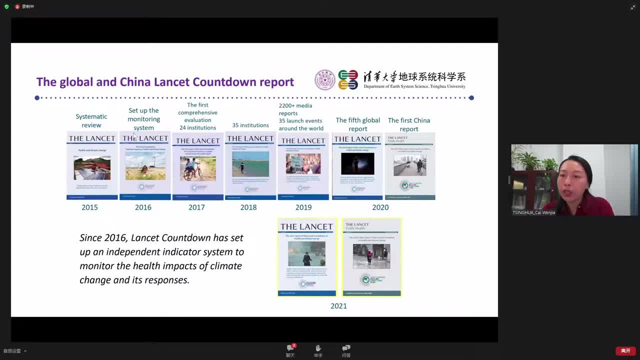 So, starting from 2017, we are using this indicator system, built in 2016, to carry out those independent evaluation or quantitative evaluation on how the health impacts from climate change is changing in every country in the world. And now we are reaching to the six of six. 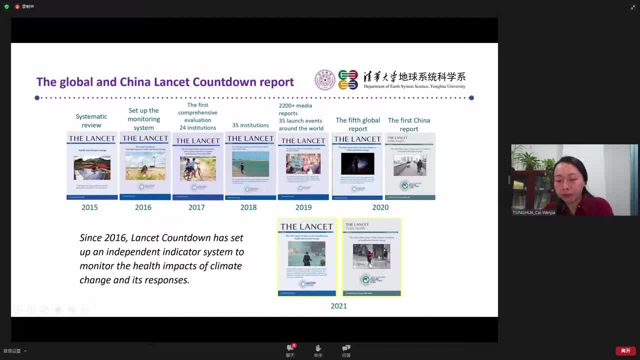 Global report and also the second China report. Actually, I am the lead author, or one of the lead author, for the China report, And we started doing it in from 2020, where, when everyone is actually locked up in their room and can't go to their offices, 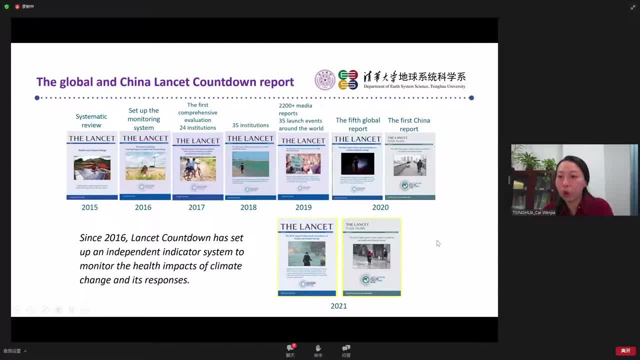 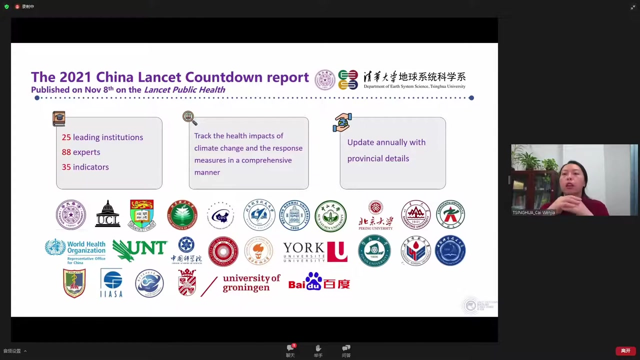 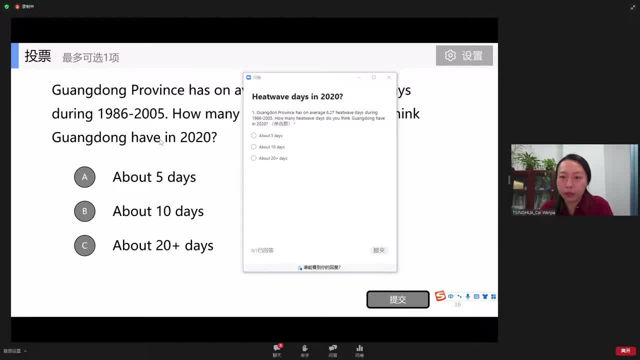 And we have set up 35 indicators which checks like the heatwave related deaths and the health impacts from extreme weather. on the pop-up window, you have 20 seconds. If you have difficulty for filling in the in the in the pop-up window, you have 20 seconds. 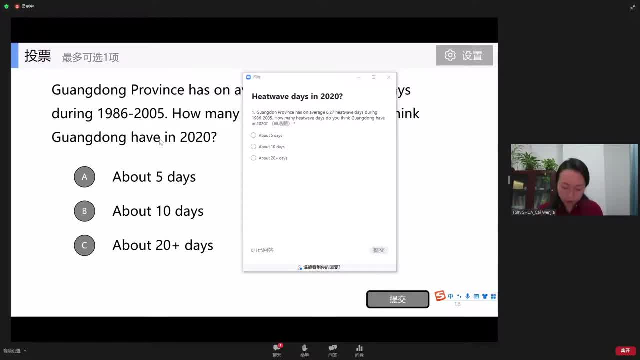 If you have difficulty for filling in the in the pop-up window. you have 20 seconds And 36 have voted for about 10 days and 2%- only 2%- have voted for about five days, And I would like to congratulate the students who have voted for C about 20 days, about 20 days. 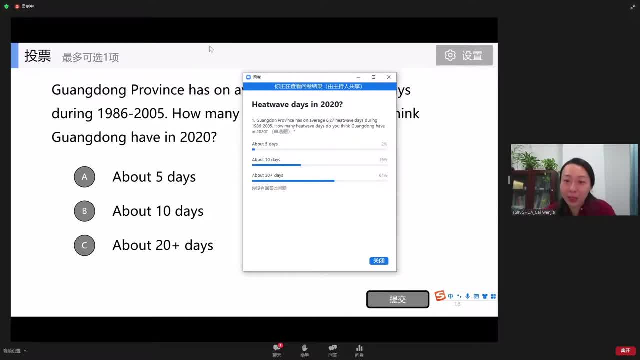 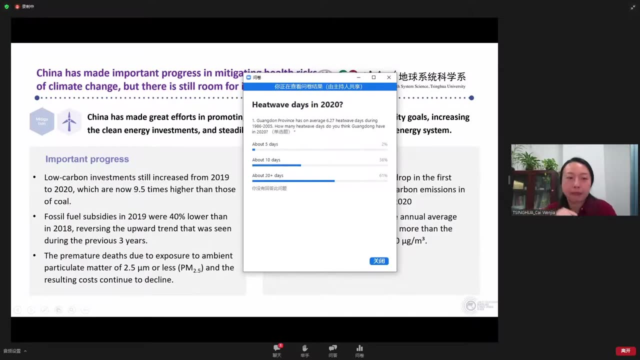 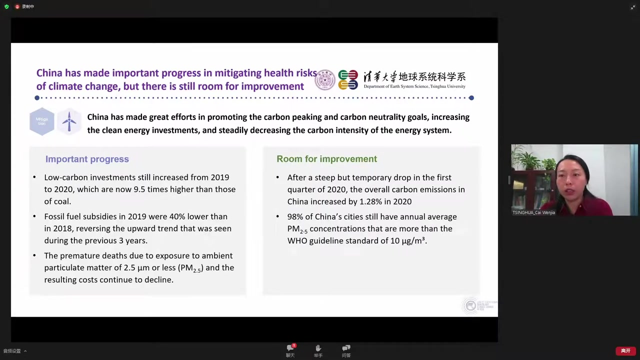 So you see how large the the growth rate is among the past during the past. Thanks for your participation In this poll And remember we will have another poll in the following slides. So in the previous slides I have talked about the health impacts of climate change. but you know we have already done a lot of work to address climate change in China and it has already had a very obvious health improvement effects. 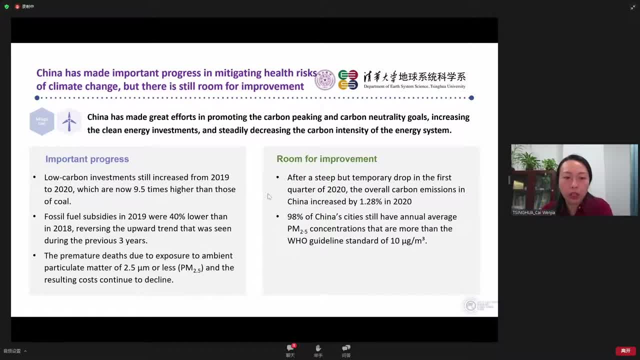 So the important progress in in China Could be seen in the low carbon investments. So, even though we had those COVID pandemic during the 2020, the low carbon investment have still increased from in the past, which are now already 9.5 times larger than those investments in coal. And also the premature deaths, Or let's say Air pollution related deaths are are continuing to decline. If you know about the health burden from air pollution in China, it is a around 1 million people. 1 million people are dying from related reasons, from air pollution and 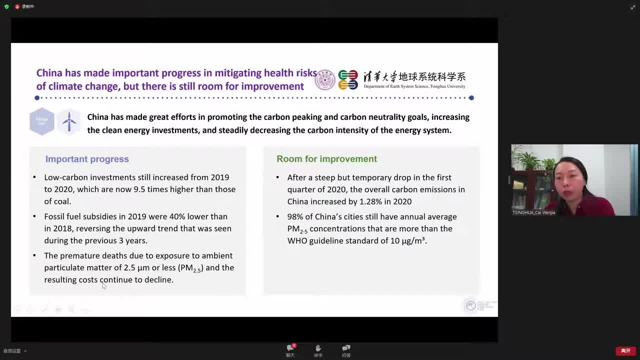 During the past, from 2013, when we had this really strict air pollution control measures In China, the death related to air pollution has decreased by 25%- 25%, which is a big improvement. but even though we have these important progresses, we still have room for improvements, for example, in the carbon emissions perspective. although we have been impacted by the pandemic in the first quarter of 2020, our overall carbon emissions have decreased by 25%, which is a big improvement. but even though we have these important progresses, we still have room for improvements, for example, in the carbon emissions perspective. although we have been impacted by the pandemic in the first quarter of 2020, our overall carbon emissions have decreased by 25%, which is a big improvement. but even though we have these important progresses, we still have room for improvements, for example, in the carbon emissions perspective. although we have been impacted by the pandemic in the first quarter of 2020, our overall carbon emissions have decreased by 25%, which is a big improvement. but even though we have these important progresses, we still have room for improvements, for example, in the carbon emissions perspective. although we have been impacted by the pandemic in 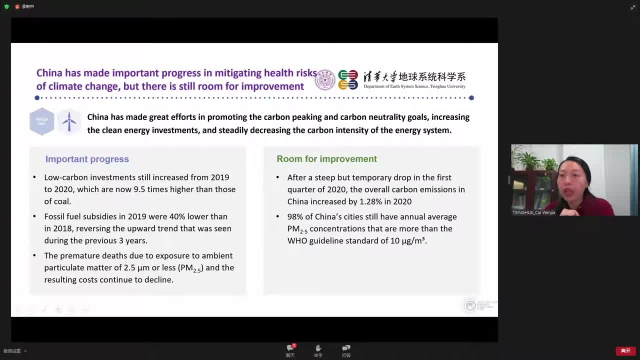 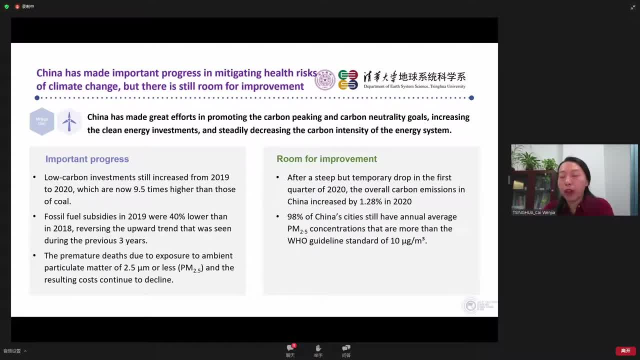 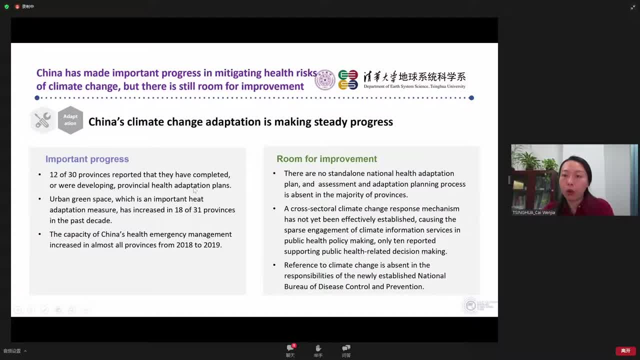 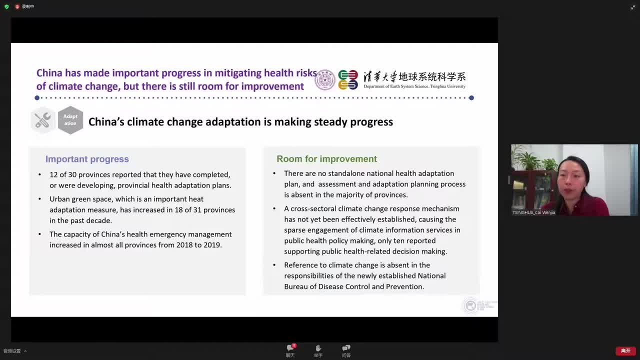 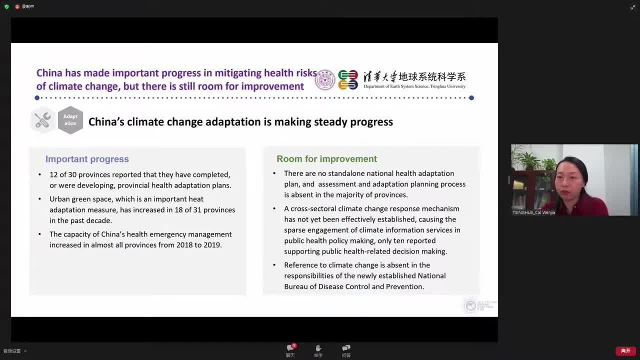 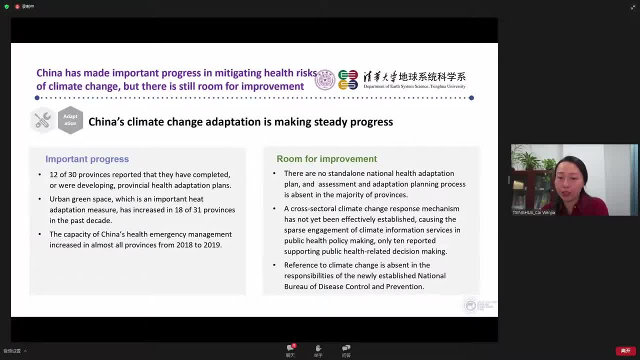 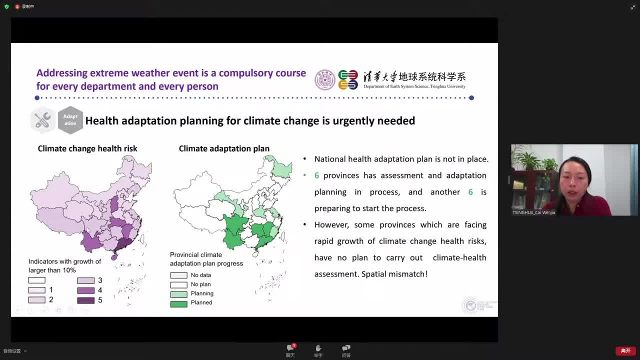 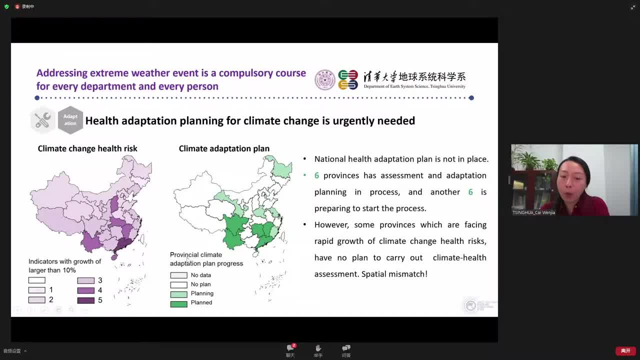 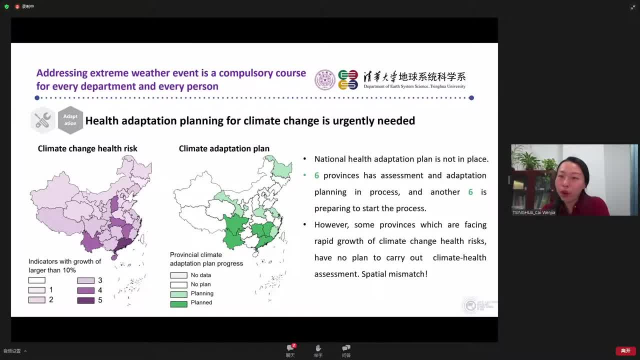 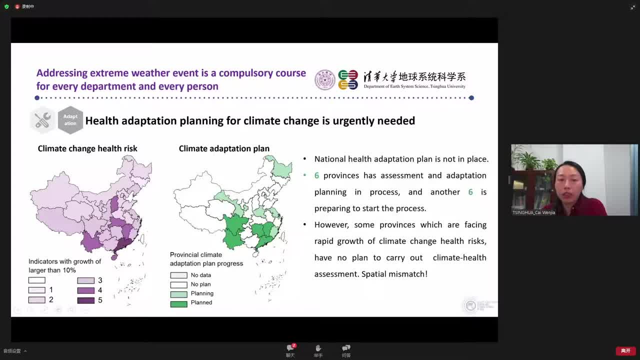 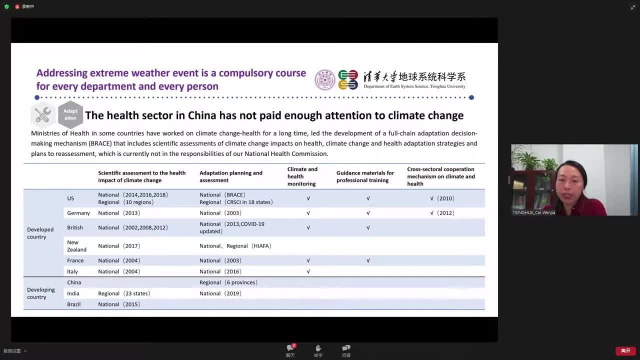 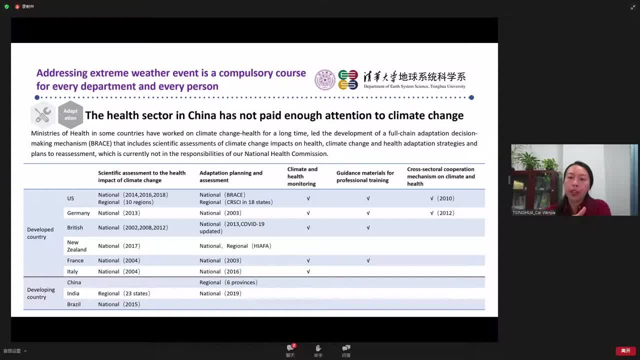 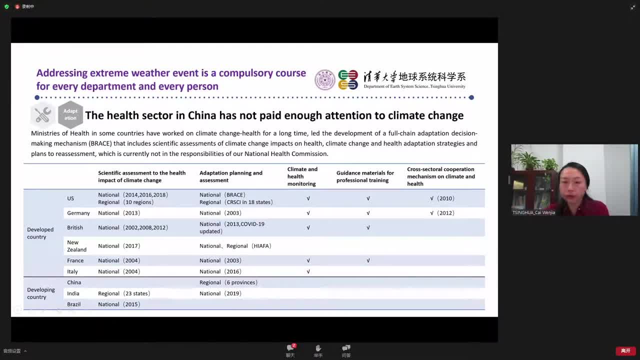 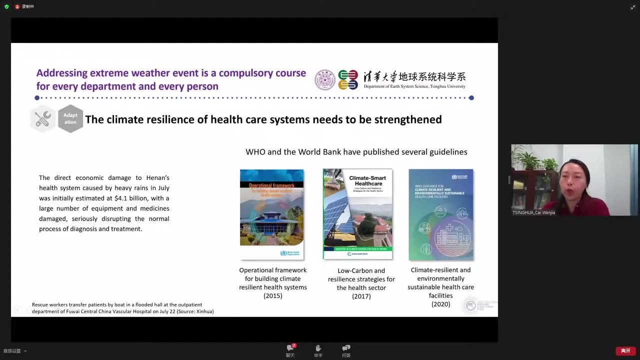 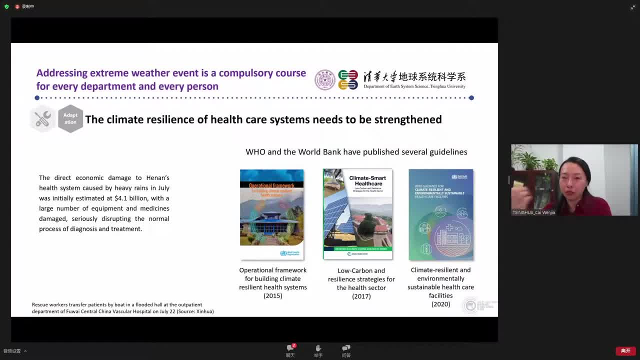 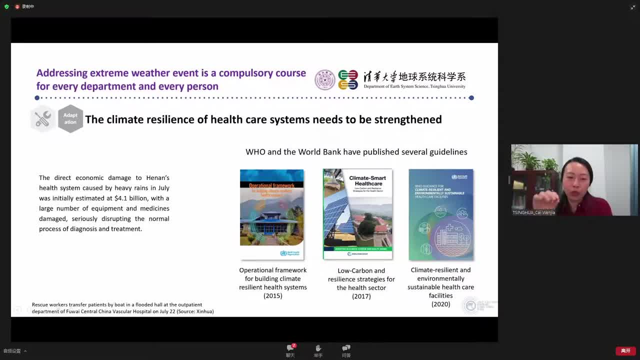 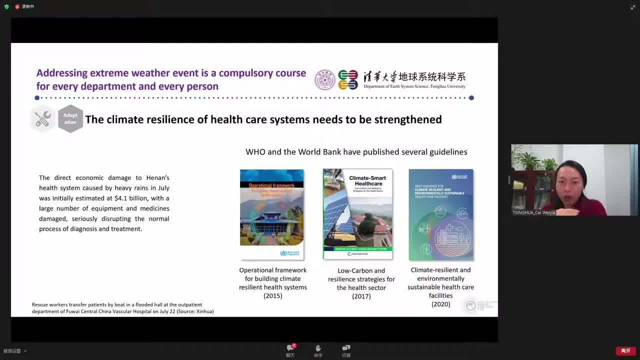 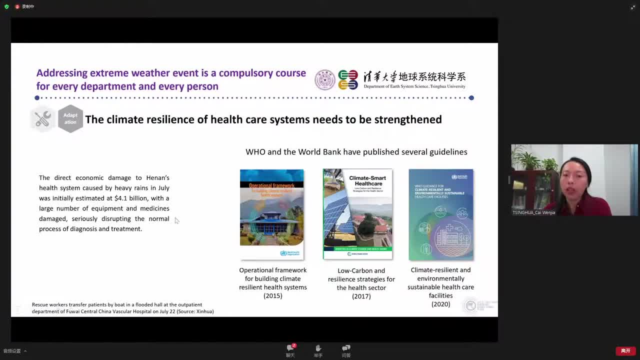 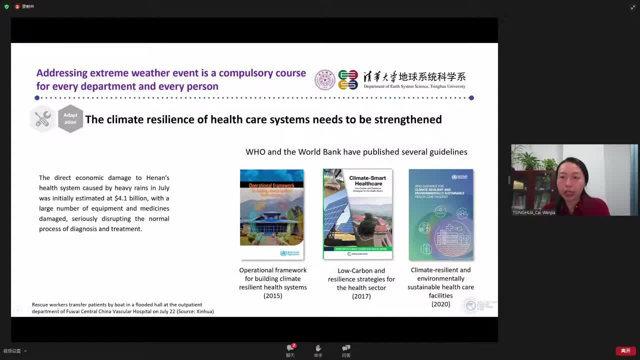 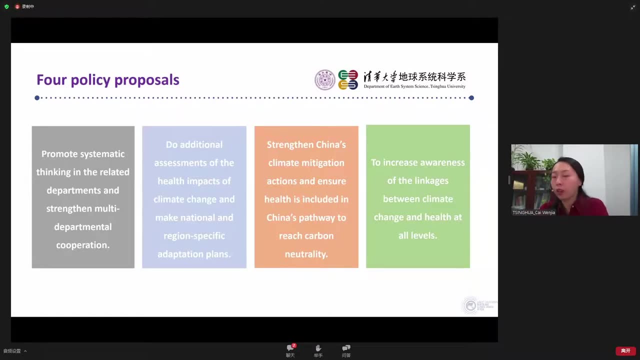 learning tools for us to read and to practice. So from the previous introduction, we have summarized several policy recommendations, such as: we need the involvement of every department and the cooperation among different departments in China, And we need to do more assessments of the health impacts of climate change and make 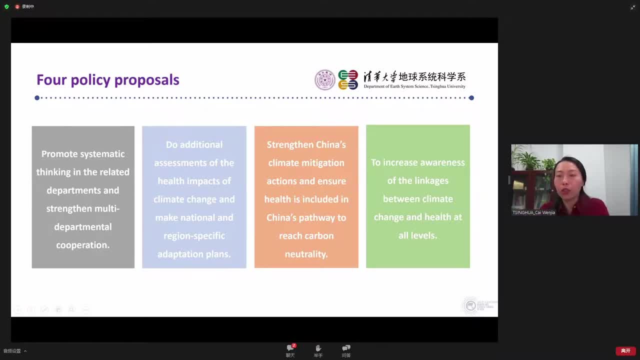 those specific or targeted response strategies for every region And we need to strengthen that. climate change and climate mitigation actions have taken into account the health impacts of climate change. So we know that these actions need to be urgent and need to be ambitious And we need to increase the awareness on this issue at all levels, not only at the public. 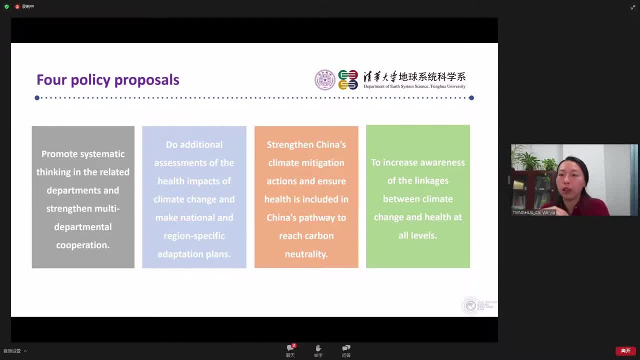 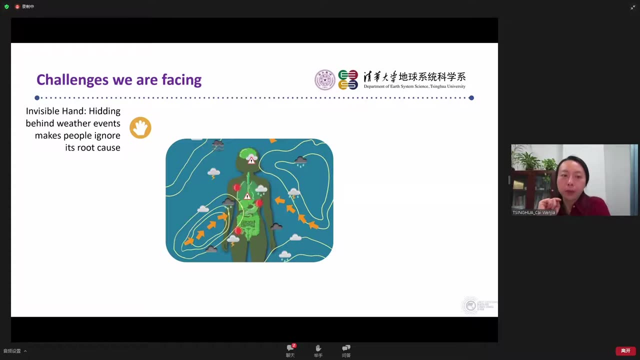 level, but also externally, And we need to increase the awareness on this issue at all levels, not only at the public level, but also externally, And also at the government, the high-level decision makers in China. So, to summarize the challenges we are facing, the first one is that the climate change is 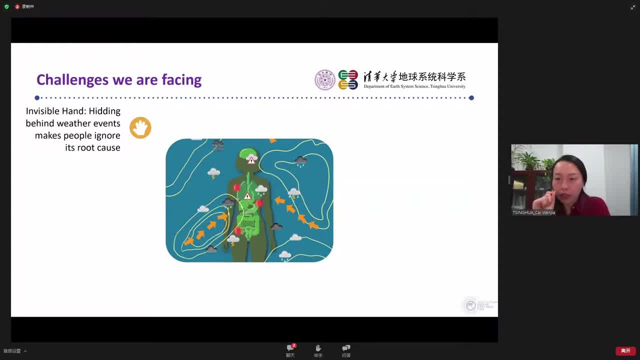 actually taking the forms of extreme weather events. So we've seen a lot of weather events in the past when we have very few or very few climate change. But as the climate change trend worsens, we will have more weather events or extreme weather events. 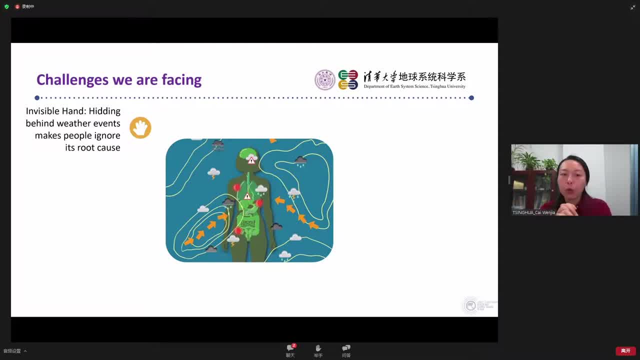 However, this climate change is hiding behind them, So that's why it usually makes people ignore what are really driving those more frequent extreme weather events. And the second challenge we're facing is that the health impacts from climate change is rising up In a fluctuating manner. 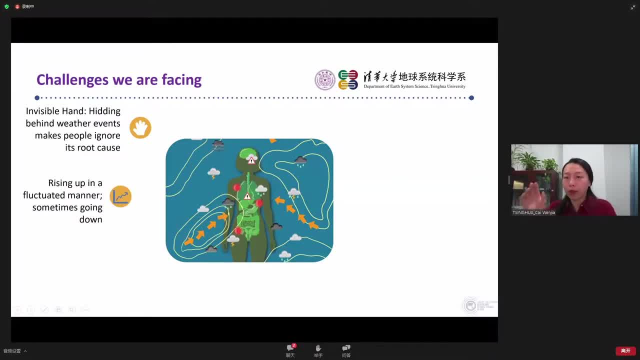 So you have seen some of the curves which I showed before about the heat-related mortality rate. So it goes up in a year and then comes down in the later year and then goes up. So sometimes people would look at this decreasing trend and starting to question whether climate 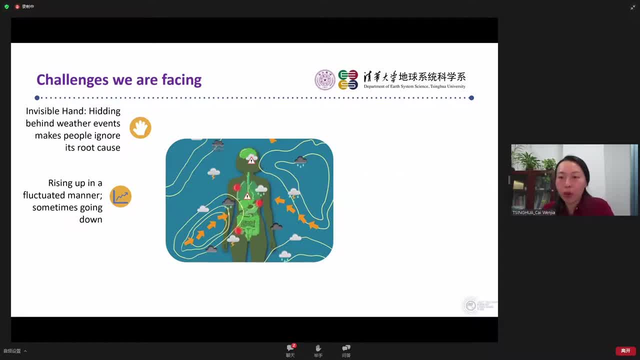 change is real, So that's also something we have been asked a lot during the communication to the common people, And we will have more and more extreme weather events that are hard for people to tackle with. And the fourth challenge is that all the impacts will be region specific. 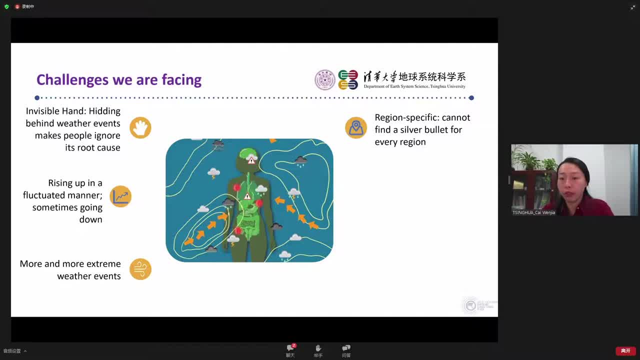 So we really can't find like a silver bullet for every region. And the fifth challenge is that some of the rare accidents for some regions will become more frequent In the future. for example, we know that typhoon usually attacks the south part of China. 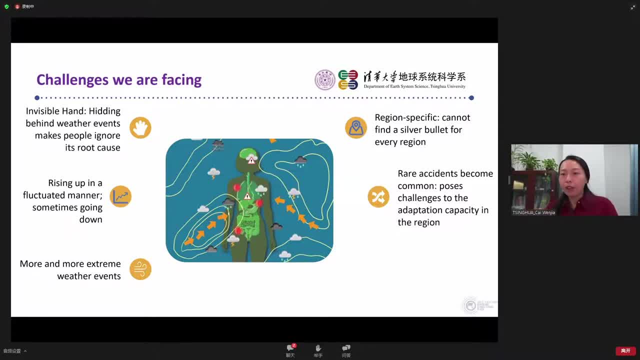 But in year 2020, three typhoons have unexpectedly attacked the northeastern part of China, like Jilin, Heilongjiang, And so in the northeast part of China, And that actually poses challenges to the adaptation capacity in this region. 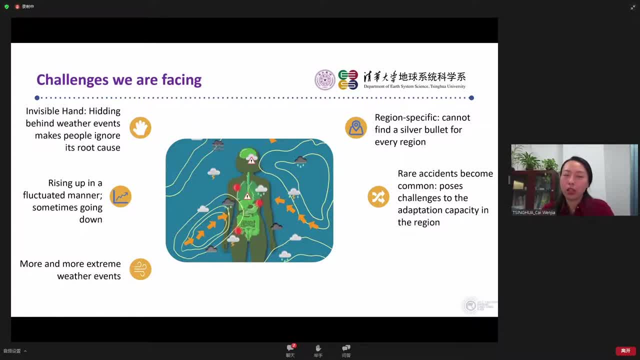 And the fifth challenges. it certainly is not the last challenges, but it's the six challenges. that I could summarize is: there are no quick fixes Because, for example, for COVID, you have those quick fixes because you can lock down the whole city and there is no conditions for the viruses to transmit. 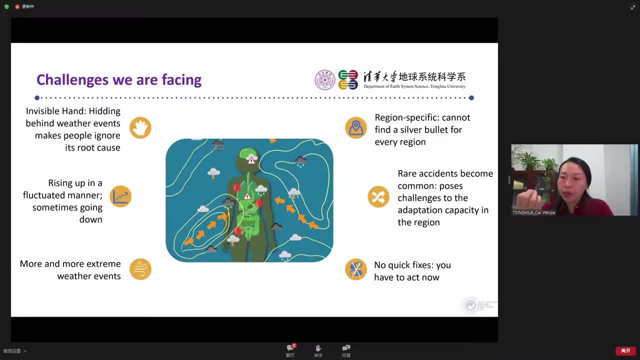 But for climate change you need to really need to act now, Because the temperature, the whole climate system has this strong inertia that you have to act now and you will see the effects in like decades. So that's something we really need to take into consideration. 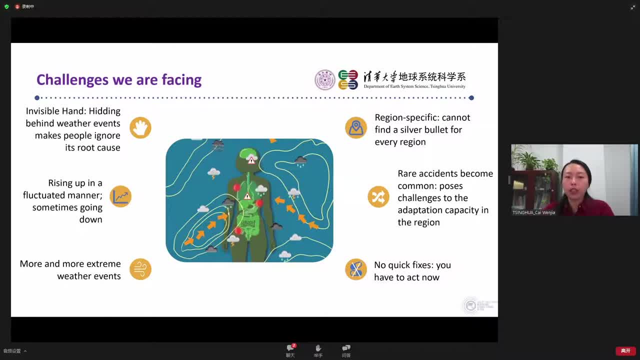 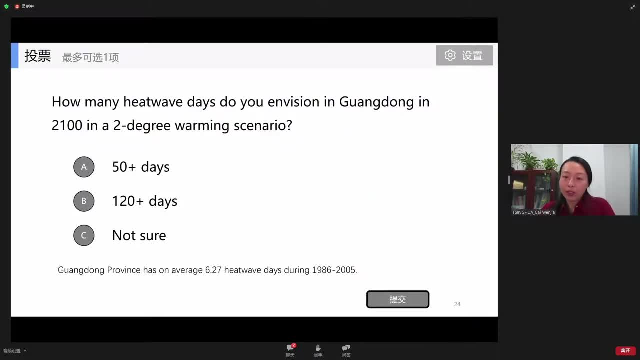 We shouldn't really delay any decisions. So here comes the second poll. So just now we know that Guangdong has, on average, six heatwave days during the past, And now we are looking into the future, assuming that we are having this two degree warming. 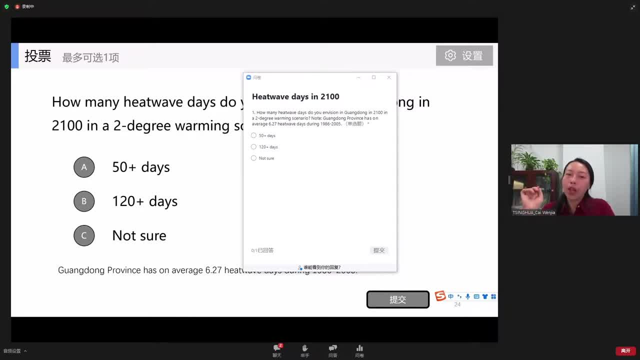 scenario. let's try to envision. how many heatwave days do you see in do you expect in Guangdong province to have at the end of the century, which means 80 years from now. So you have three choices. More than 50 days. 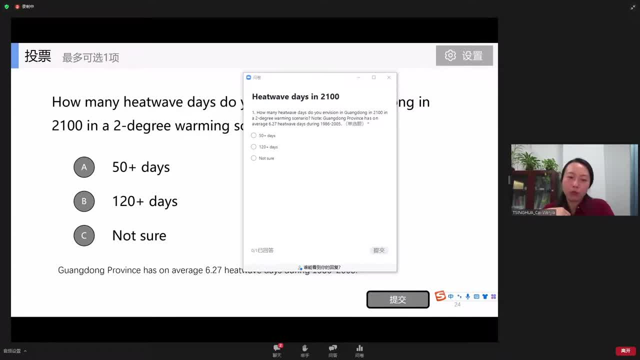 More than 120 days, Or if you're not sure, you are certainly allowed to vote for not sure. So you have 20 minutes for sorry, 20 seconds to answer the question. But if you're not sure, or you don't have an answer or you just feel like you've taken. 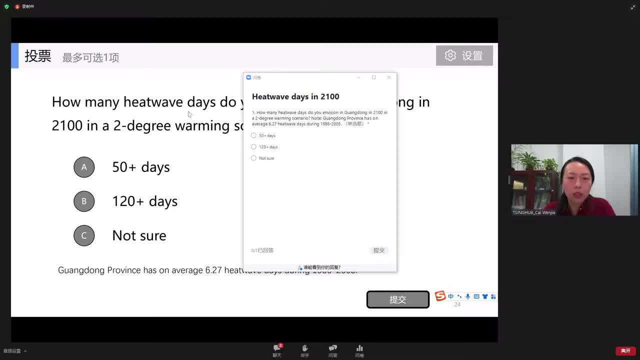 your own decision. Let's go with you. Let's make sure. 13 seconds, All right. So we are good, Let's see. All right, I can see all the members and we don't really have a lot of time left. 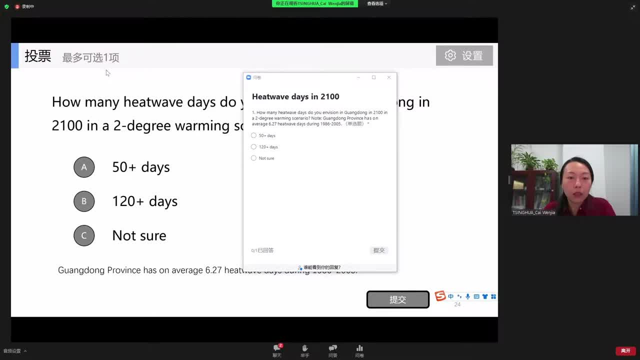 So let me do a quick poll then. Okay, So the question is: do we have an opportunity to visit Guangdong, To visit? Let me do a quick poll here. So our first poll: we're looking at, we're looking at, we're looking at five different 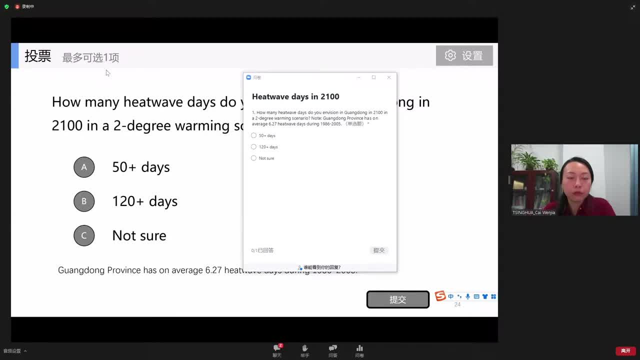 different cities in Guangdong And we have at least six days free investment. So we're looking at about 6,000 miles of spending. Well, interestingly, about 34% of participants today voted for more than 50 days and more. 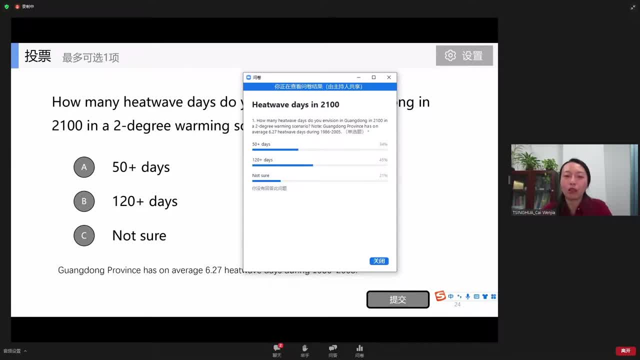 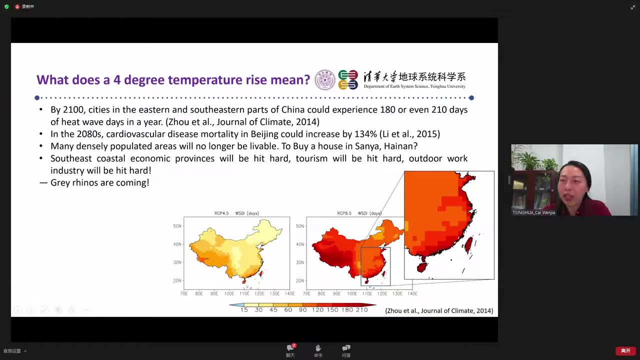 than 40%, voted for more than 120 days And let's together see the magic ball. So we have this projection studies that have been done widely in China and it shows that by year 2100, some cities in eastern and south part of China, they would experience more. 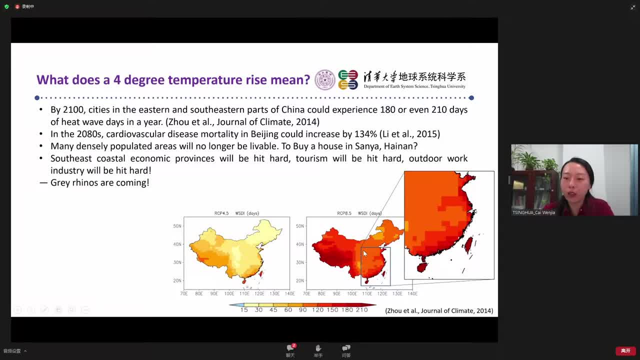 than 180 days or even 210 days of heatwave days in a year. What does heatwave days mean? Well, although it means different definition or different definition, Different conditions for different regions, But usually we could say like continuously three days, with the daily temperatures higher. 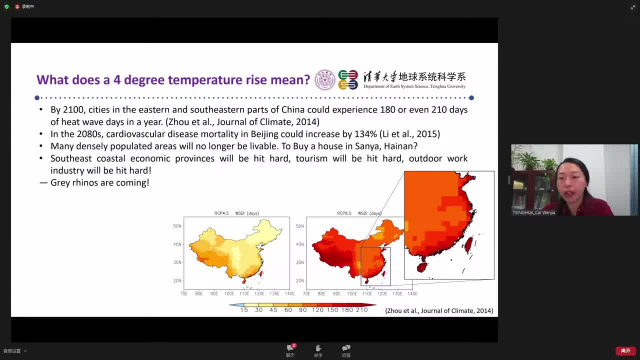 than 35 Celsius degrees. we could define it as a heatwave days. So can you imagine living in the city where half of the year, you are staying in such a high temperature? And just now we mentioned that there is the two degree warming scenario, which are shown. 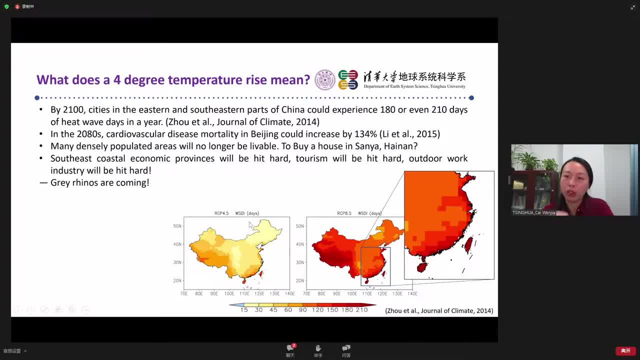 here the RCP 4.5 scenario, which is about two degrees. So you can see, in Guangdong province, some parts of the province will have more than 180 days more heatwave days and if we don't do any climate action, we are aiming for the. 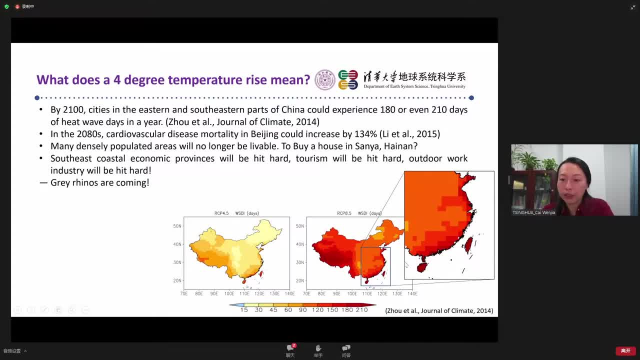 RCP 8.5 scenario. Yeah, Okay, you see, a large proportion of China is covered by this deadly red color, So the future will look very similar to what I have just mentioned, not only from the heat wave- sorry, the heat related excess mortality. 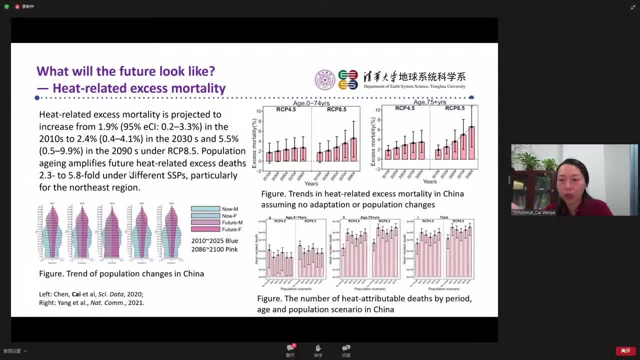 that are increasing rapidly, not only because of climate change, but also from the population changes, which means we're having a really strong aging trend, And also, if we look at the high temperature subsidies, it is something that we are paying for those workers. 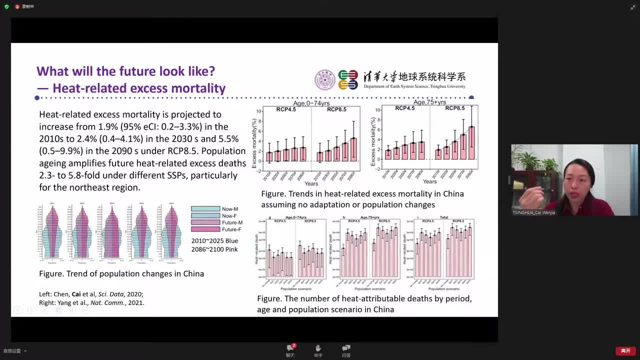 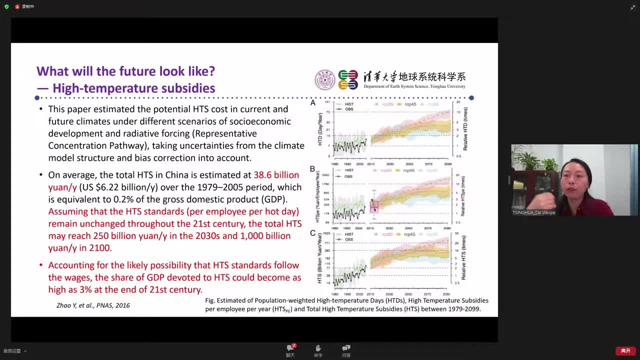 especially outdoor workers when they are working in the high temperature conditions. So it is requested by the government to pay for this outdoor workers a certain amount of money to subsidize their like health outcomes Under the high temperature situations, And this study is published in the proceedings. 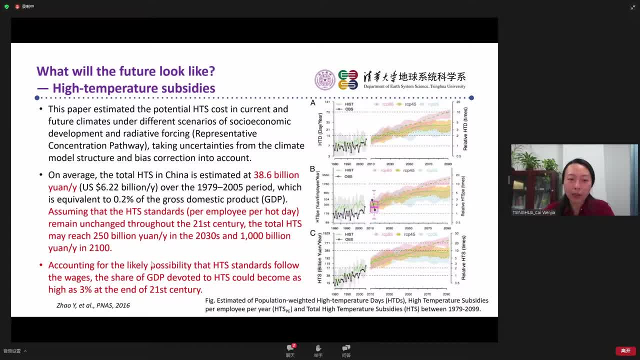 of National Academy of Science in the United States have estimated that the share of GDP devoted to high temperature subsidies- subsidies- could become as high as 3% at the end of the 21st century. 3%, we are actually like investing a similar amount of GDP. 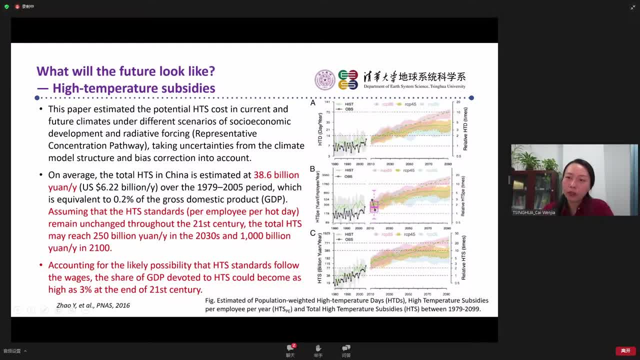 into education. So it's a very, very important thing. It's a very, very important thing. It's a very, very important thing. So you could see how large these amount of high temperature subsidies would go to. So the final part of my presentation would be linked. 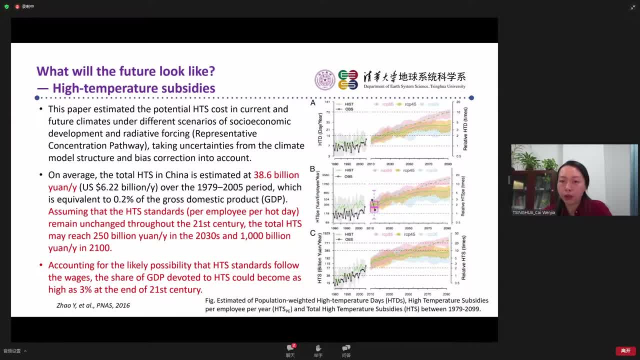 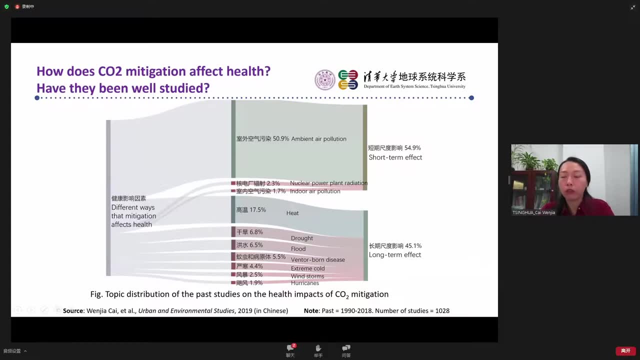 with how does mitigation affect health? And there are actually a lot of channels that mitigation could affect health. For example, something we're most familiar with is that mitigation usually requires the phase out of fossil fuels, So the reduction of coal use, the oil consumption. the natural gas consumption and that all leads to the reduced air pollution levels in this country. So by reducing air pollution that will have very immediate health impacts to improve health, But also in the long-term perspective it could help reduce the high temperature days. 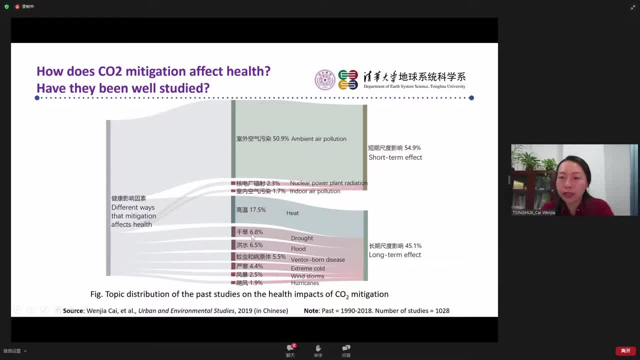 such as the heat wave days, and also reduce the frequency and the intensity of flood and drought and cold spell and hurricanes. So these all belong to the long-term effects And a lot of people, a lot of the current literatures, are focusing on the air pollution. And many modeling studies have shown that the health risks or, sorry, the health co-benefits from reduced air pollution would outweigh the mitigation cost would outweigh the mitigation cost, And in China it is especially so because in our study we have estimated that in 2050,. 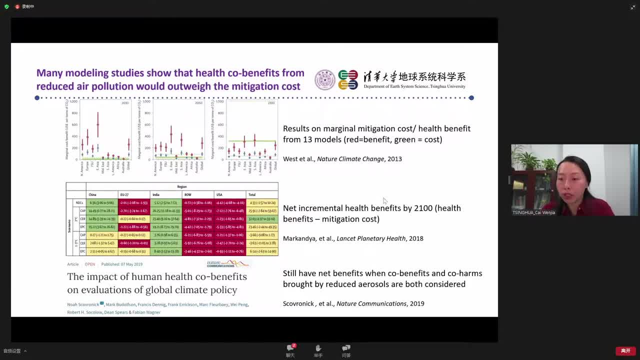 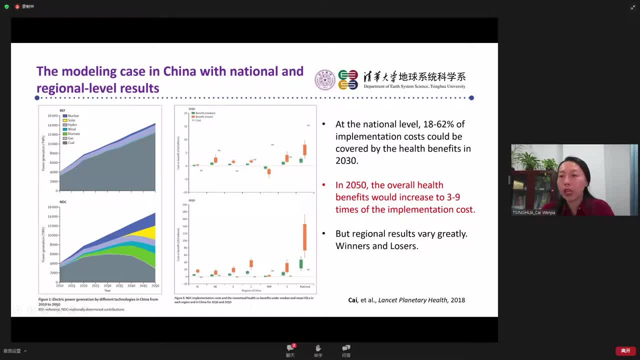 the overall health benefits would be equivalent to three or nine times of the mitigation cost. So it means all the mitigation costs could be offset by the health co-benefits. And there are other ways that mitigation could affect health, For example to reduce. 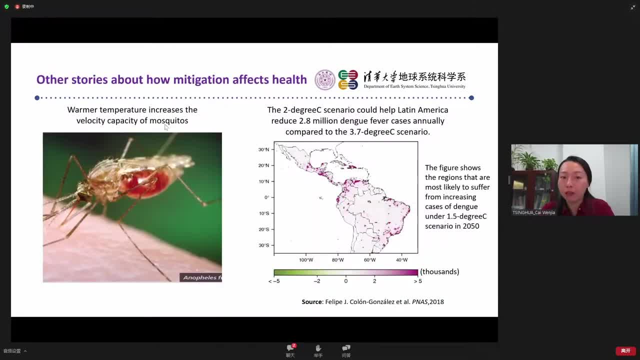 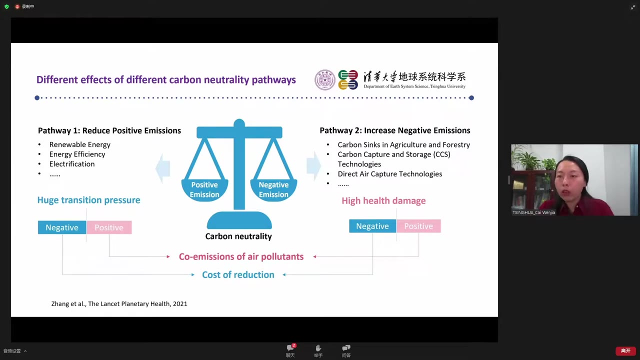 the vectorial capacity of mosquitoes And this graph showing how many less dengue fever cases would be happening in Latin America in the less warming scenario. So we all know that China has published this carbon neutrality goals in 2020.. And in this study that we published over this month, 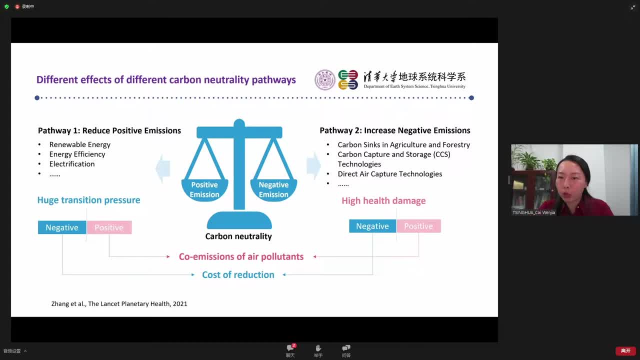 we have explored how the carbon neutrality pathways would impact human health, And this is actually belongs to the short-term health effects from climate change. We modeled how the climate neutrality goal would help reduce the air pollution in China and then leads to health benefits in China. 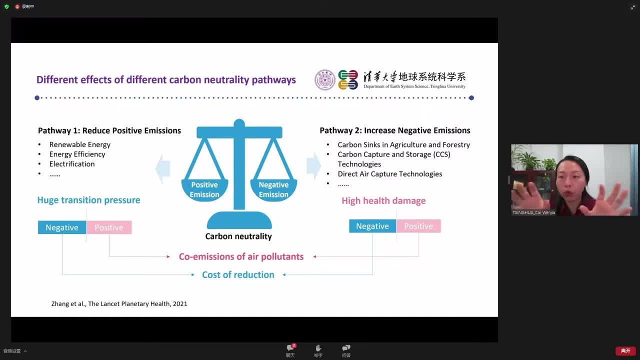 But in this study we have innovatively explored two different models, different pathways to realize carbon neutrality pathway, carbon neutrality goal. The first one is we could try to use more renewable energy to reduce those so-called positive emissions, because we know that carbon neutrality means. 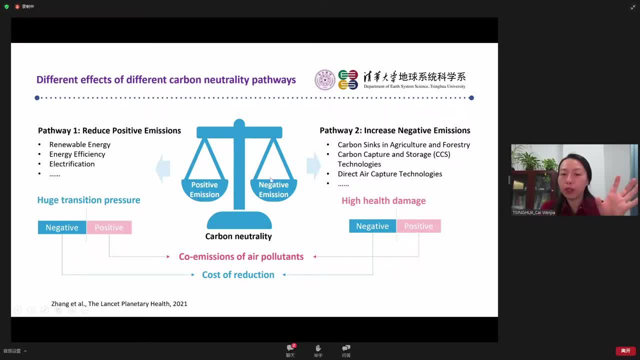 that the positive emissions could be reduced by the negative emissions. So they achieve like a balance. But the other pathway is to increase those negative emissions which we use, for example, the biomass or the agriculture or the forestry management tools to increase the carbon sinks in the current climate system. 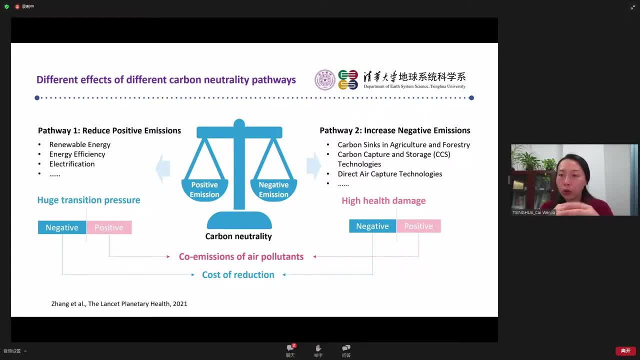 Or we use carbon capture and storage to storage these emissions from the atmosphere. So they have actually trade-offs. So the first pathway, they are encountering huge transition pressures Or huge transition costs Because we know to use renewable energy to replace the current fossil fuel. 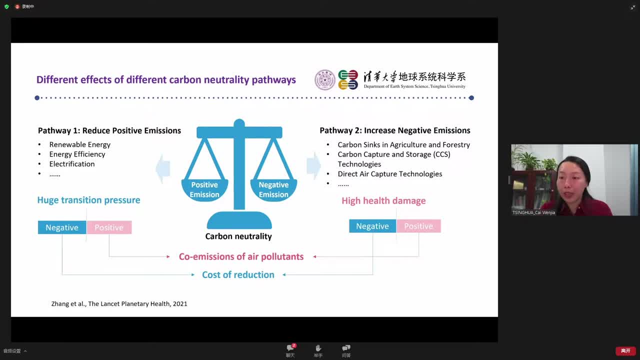 we need to close down a lot of plants in China and to force them to use new technologies, And that will cause a huge amount of cost of emission reduction. However, if we let them stay as what they do right now, we need to use more negative emission technologies. 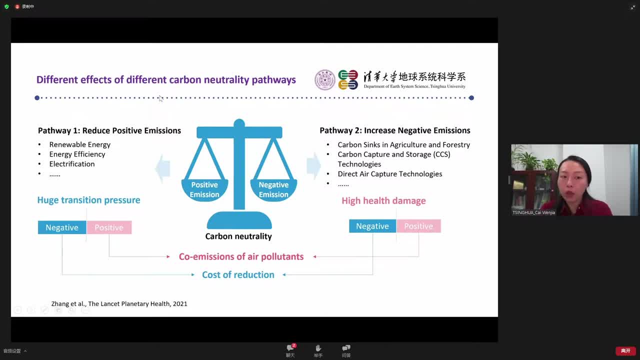 to offset their emission, But in that way we will allow them to continuously emit those hazardous air pollution. So that will emit more air pollution than the. that will emit more air pollution. So that causes health problems. So in this study we want to find out: 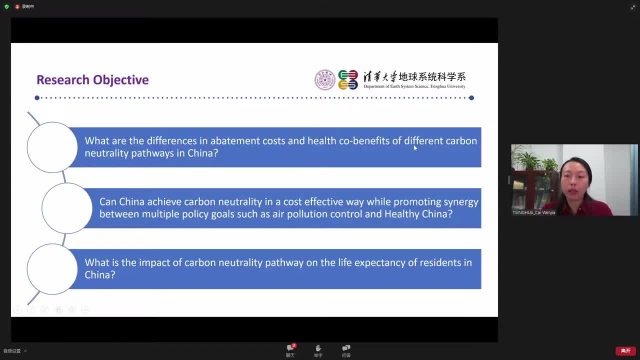 what are the differences in the abatement cost and health co-benefits of different carbon neutrality pathways in China? and also because all the previous studies they have estimated, like the, they are describing the health co-benefits of carbon mitigation as the 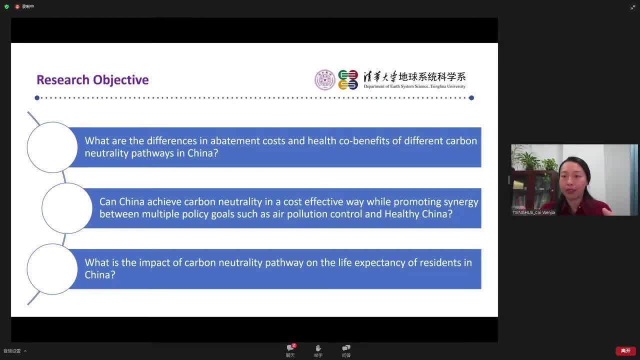 like the reduced deaths from the carbon mitigation. So we could say like 1,000 people well are saved, have been saved. Their lives have been saved due to the mitigation actions. However, it's really hard for common people to understand. 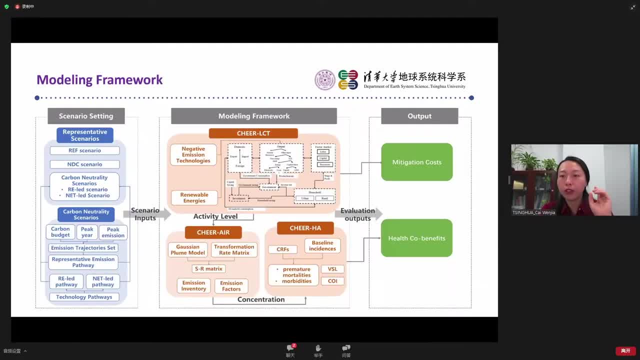 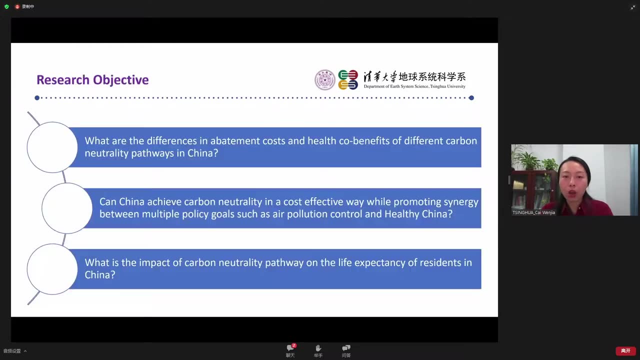 So we have in this study, we have innovatively changed, interpreted this number to the impacts, to the life expectancy of the average people. So that is something we're doing in this, innovatively, in this study. So I will go directly to the results. 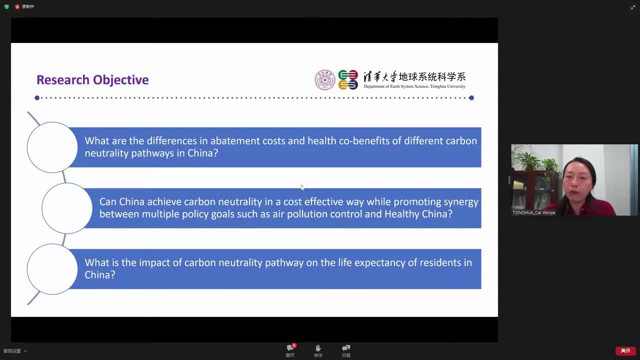 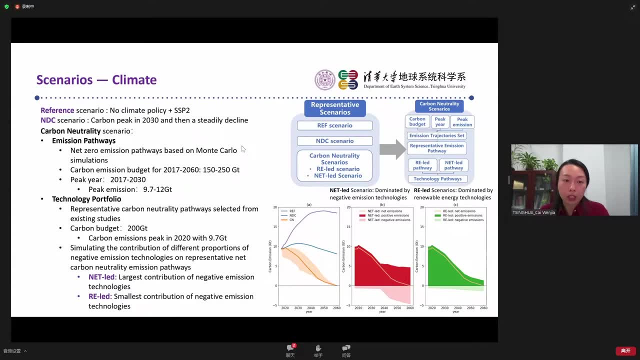 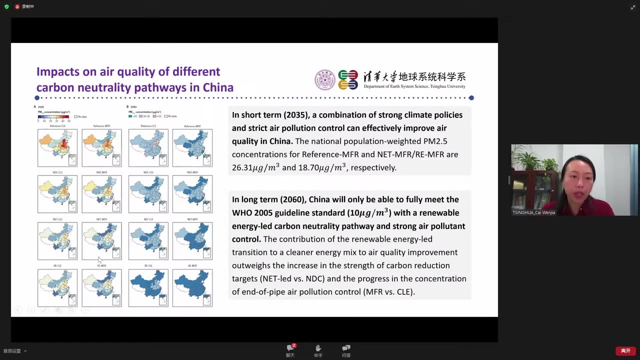 So in short term, if we combine the climate policies with strict air pollution control policies, we could effectively improve the air quality in China. You can see from this figure, this is- these two columns- shows the 2035 air pollution level And these graphs shows the 2060,. 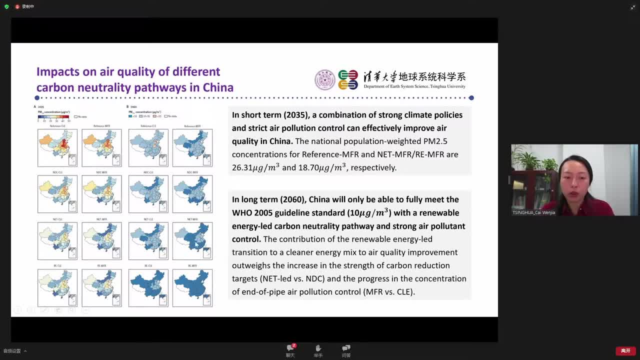 the air pollution level in the 2060.. And a lot of the regions are less than 10, less than the WHO's recommendation level or the guidelines standard. So in the long term the effects will be much obvious And we have also calculated the related mortality. 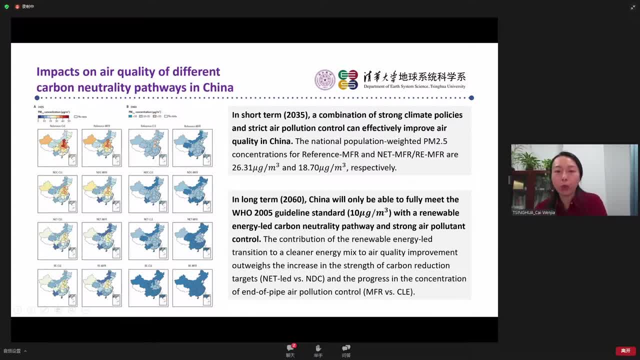 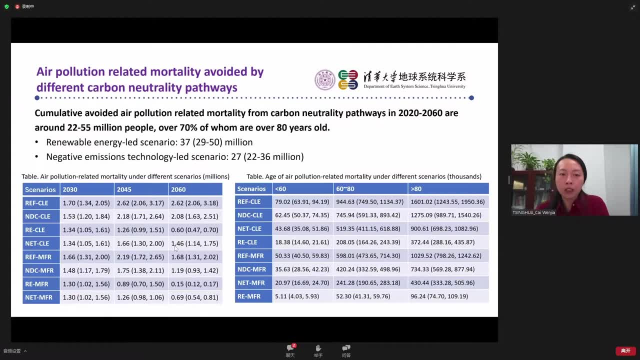 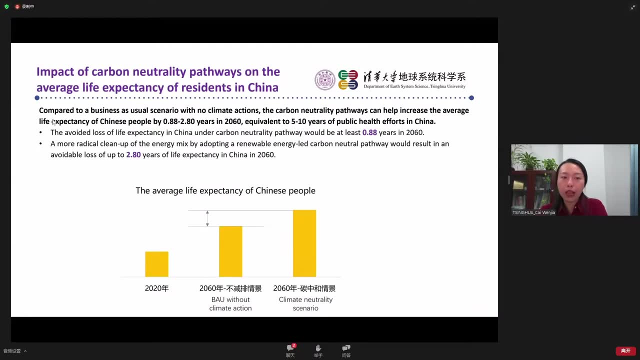 which used to be shown by the previous study, But in this study we have shown, as I just mentioned, the impact on the average life expectancy of residents in China. So we our findings shows that the carbon neutrality pathway could help increase the average life expectancy. 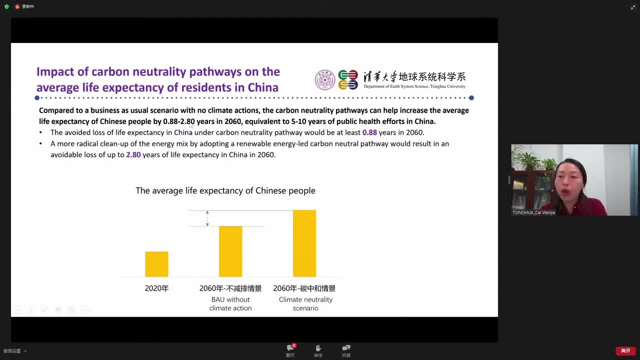 of Chinese people by almost one to 2.8 years in 2060.. So what does it mean? one to three years of life expectancy increase, It is equivalent to about five to 10 years of public health efforts in China. So if we asked that the National Health Commission 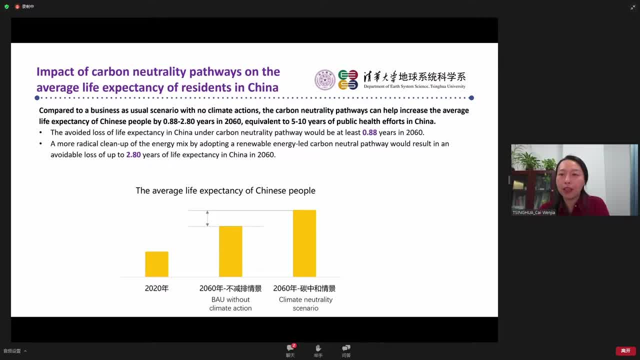 to improve the life expectancy for Chinese people by one year, it will take them almost five years to finish, so So it shows how large the carbon neutrality is improving people's health in China, And that implies that carbon neutrality is something that relates to each one of us. 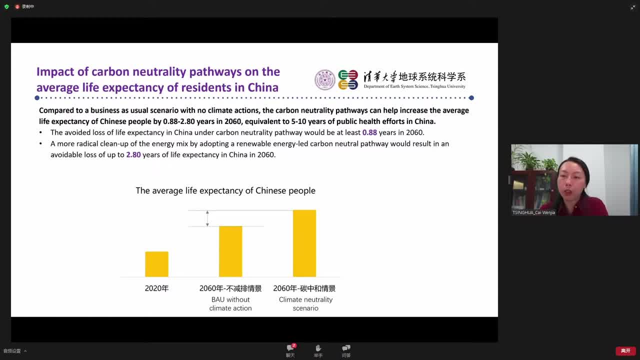 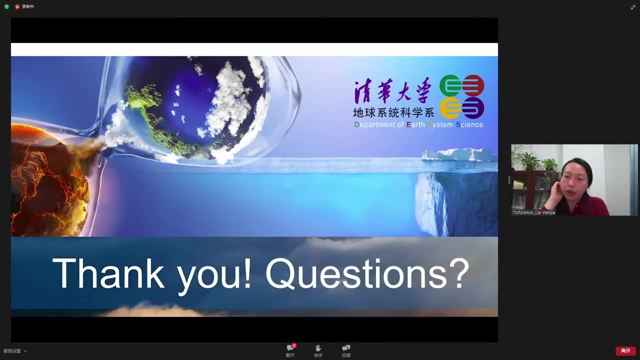 And if we can help with the carbon neutrality goal, we will finally benefit from them. So I will stop here and that's my presentation about the health impacts from climate change and carbon neutrality, And I also want you to remember that our health is closely related to the climate change trends in the world. 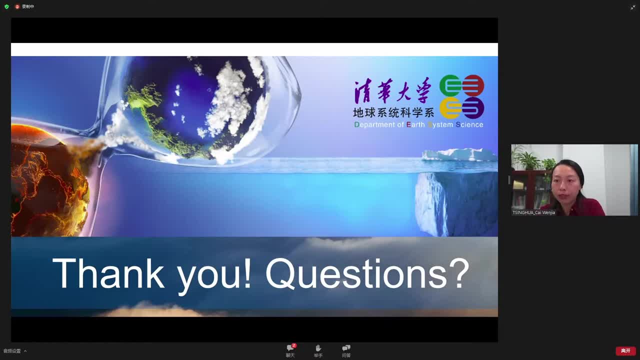 and also in the region that you currently live in, And if we could help with reducing carbon emissions and that will finally leads to the health co-benefits to every one of us, and not only to you, to your parents and especially to your children. 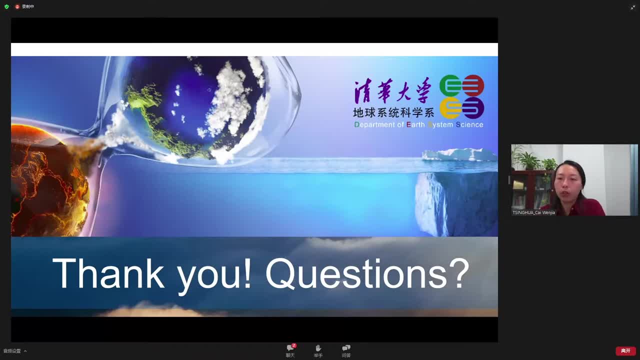 So we really need to work together to help achieve that goal. So that's the end of my presentation And I really thank you for your participation and attention for this course, And then we will have these discussion session. So now I would like to invite all of you. 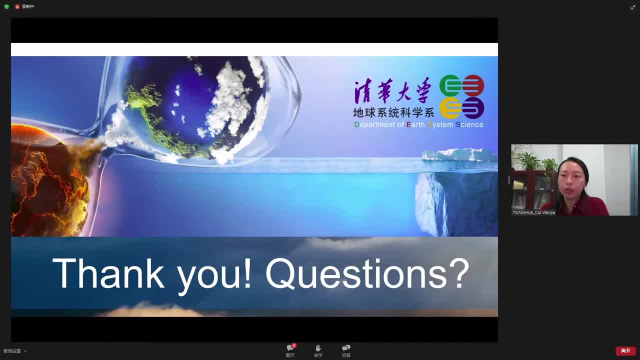 if you have any questions in mind, don't be shy to ask your questions, And if you can open your camera and to ask your questions directly, that's even better. So I would say: maybe some of you have questions, Maybe you need to prepare something for your. 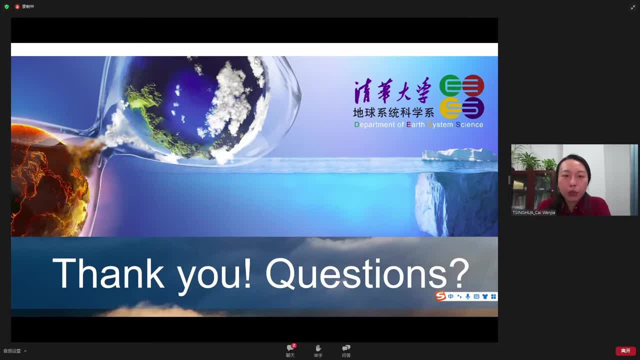 prepare some time for your questions, But I see two questions in the chat box. Let's start from the earlier one, If you could recommend. so it's raised by Erica. So she said if it's a she. sorry if I'm wrong. 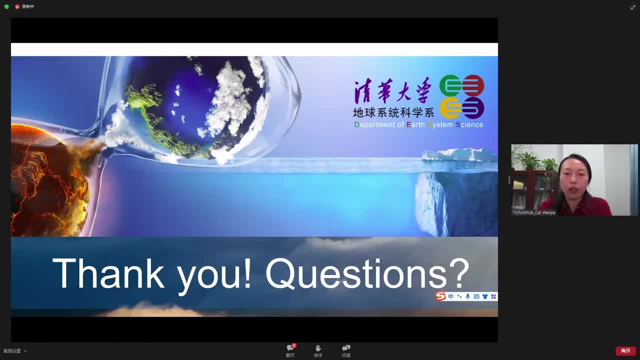 if you could recommend only one change to our lifestyle to help reduce the detrimental effects of extreme weather, what would you propose? That's a really good question. I mean changing our lifestyle. you can't really reduce the incidence of extreme weather. 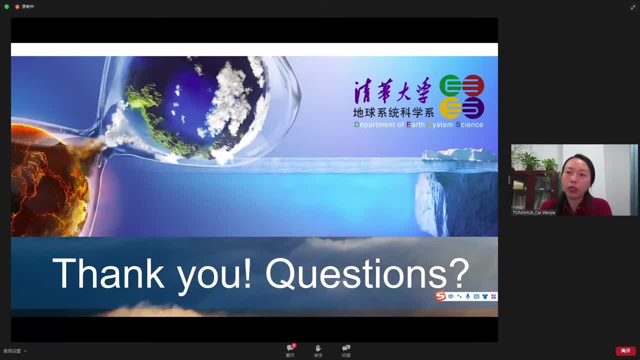 It's well if we do, really, if we make joint efforts to reduce the emissions, that will help reduce the effects of extreme weather. And if you would say, one change to our lifestyle- it's hard to name just one, but I would name two if you allow me. 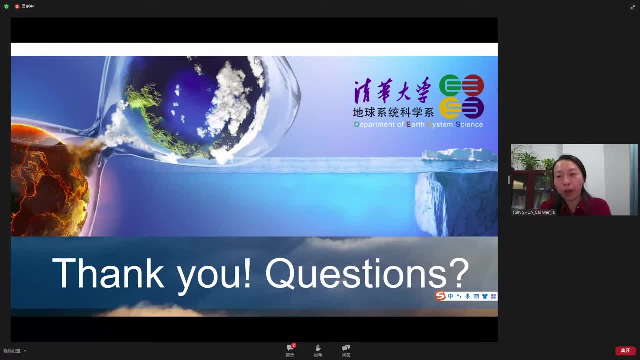 So the first one would be using more public transportation to reduce our transportation related emissions, because you know a lot of well around 20% or 15 to 20% of emissions in China and even a larger share of the emissions. 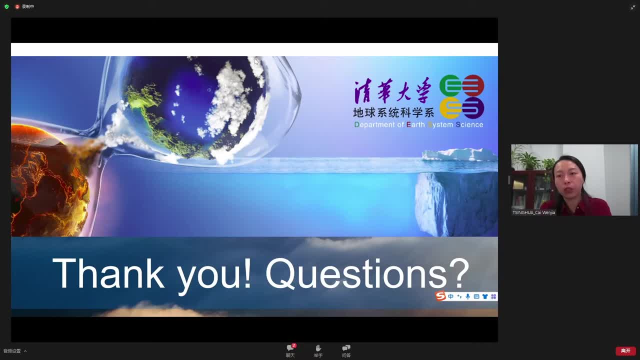 come from the transportation sector in developed countries, So that would be something that each one of us could involve in. And the second one is to reduce our emissions, is to reduce the food waste, Because just now we only focused on the carbon dioxide. 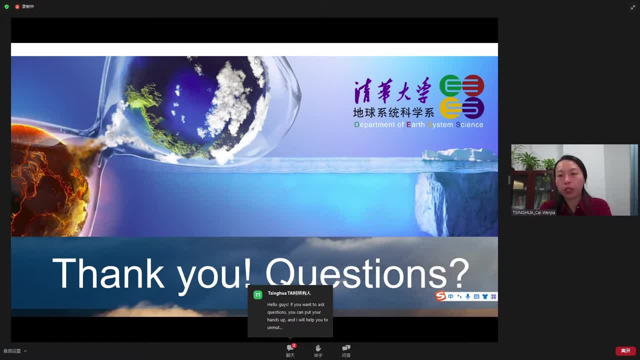 emission reduction. but you know, the food production and also the food waste also contributed a large share to the global emissions. So that's something we could easily do. But another part of the coin, or another side of the coin, is that imagine that we still have this global warming trend. 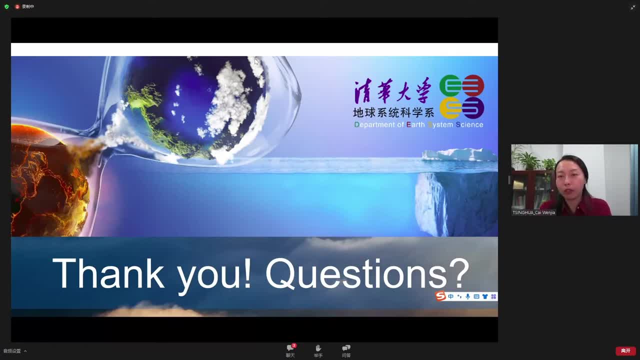 and we want to reduce the effects of extreme weather events. Actually, I'm suggesting everyone to prepare better skills to rescue yourself from those extreme weather events. If you are driving a car during the heavy precipitation, you should be aware that there are some regions. 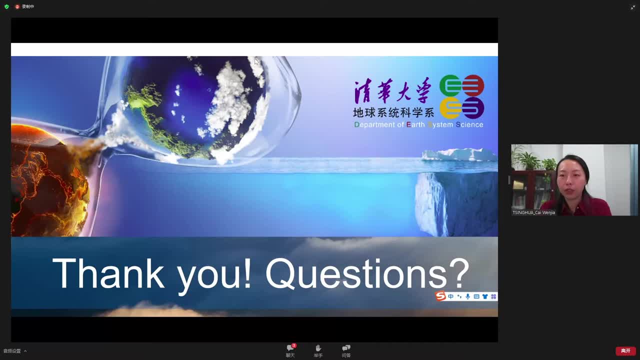 or some roads or some areas that you should never go to because they are low, having low latitude, and they are easily to be buried by water. And if you are at home and sometimes you can prepare more food and the vegetables to prepare any unexpected extreme weather events. 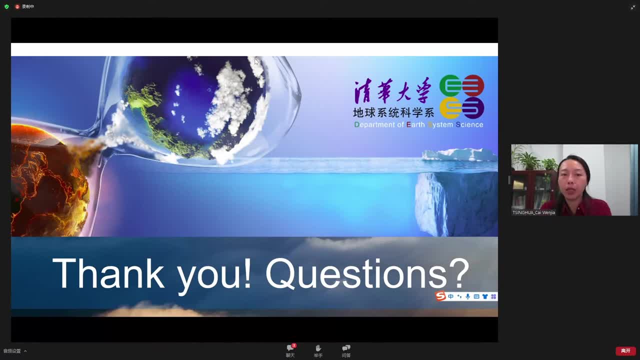 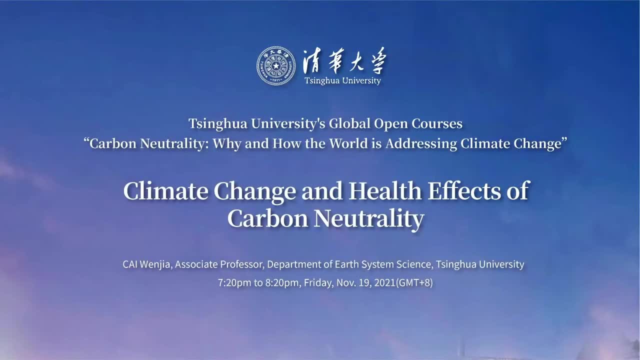 And that's something we are, we have been, And it's a really good way for us to take this opportunity to think about how we can also help the world. Thank you, Thank you, Scott, Thank you, Thank you, Thank you.